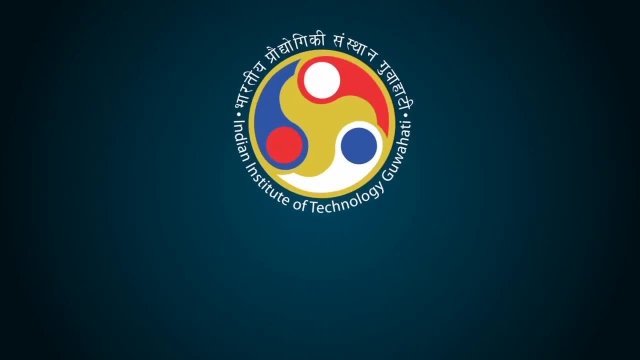 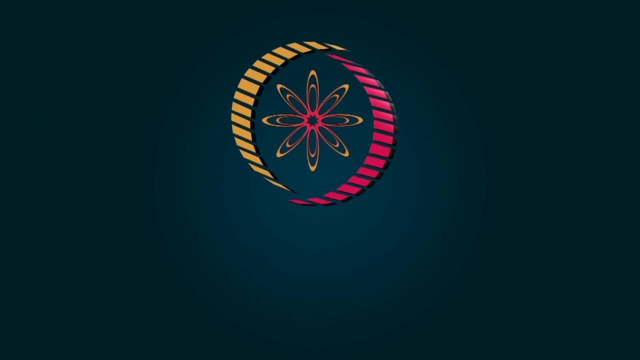 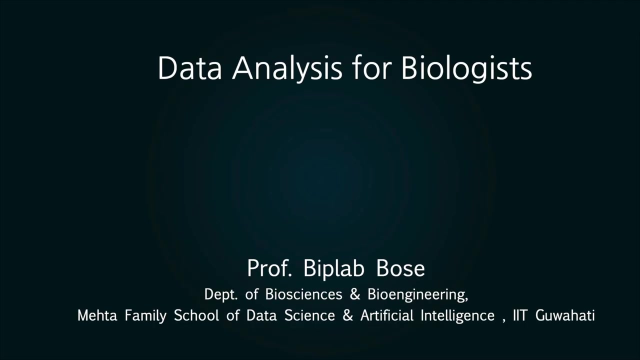 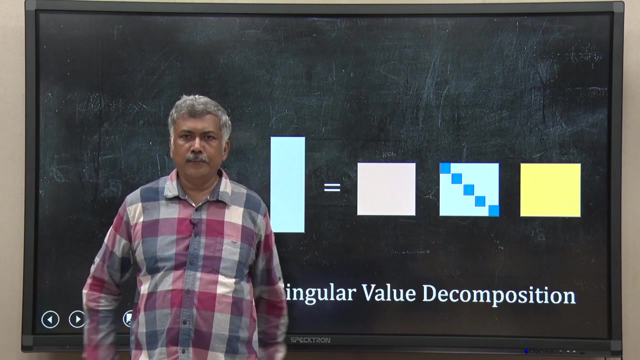 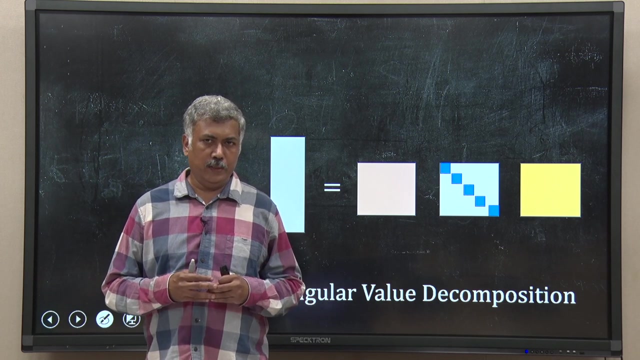 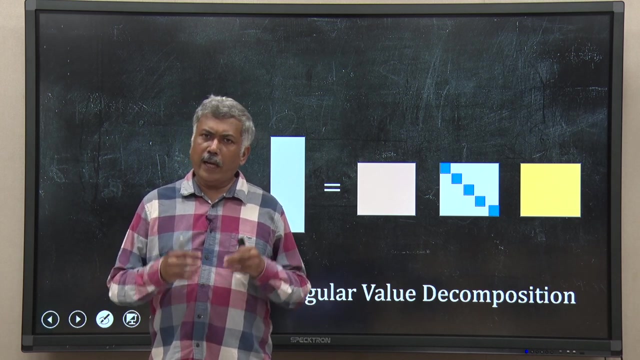 Thank you for watching. Welcome back everyone. In this video we will discuss about singular value decomposition. It is a very powerful technique of linear algebra which is widely used in data analysis and machine learning. But I will start discussion with a different decomposition That is called 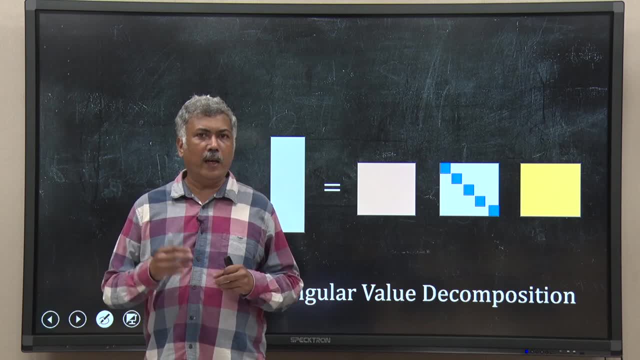 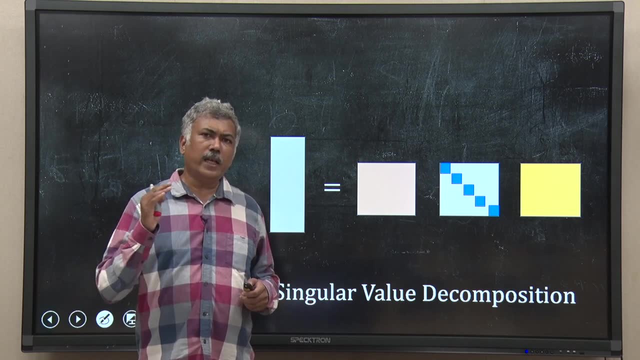 eigen decomposition And we have studied eigen value in one of the lecture in this series of linear algebra talk in this data analysis course. So let me start with what is the eigen value decomposition, What is the eigen value and what is the eigen vector? So, if you remember, if I have a square, 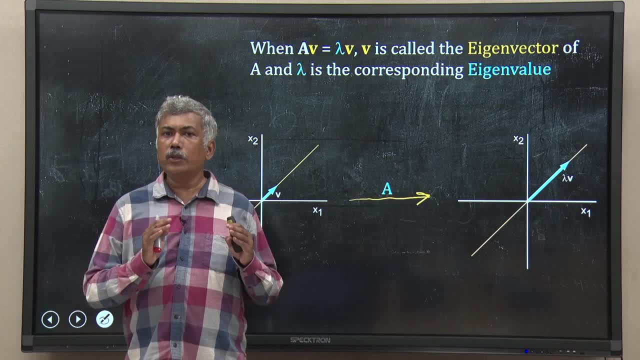 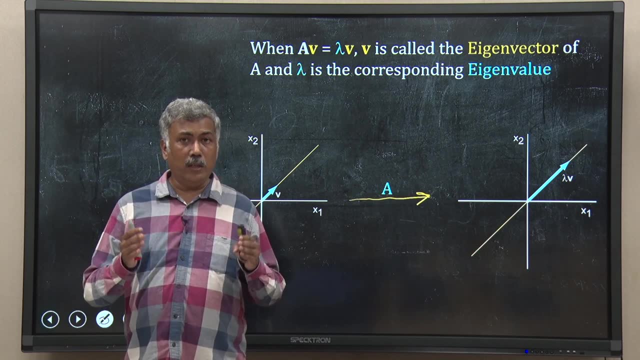 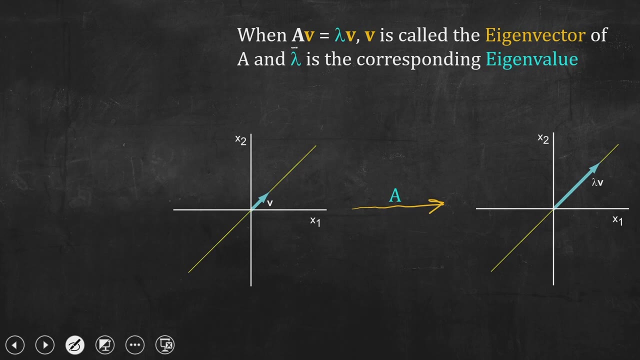 matrix. remember eigen value. eigen vectors are defined only for square matrix. So if I have a square matrix, A and then its eigen vector is called V and the eigen value corresponding eigen value is lambda, is such that if I make A into V, the matrix into the vector eigen. 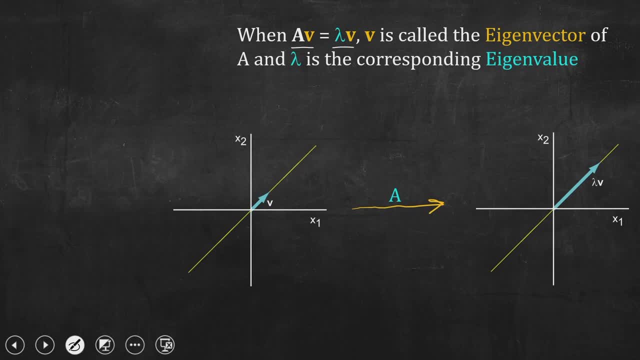 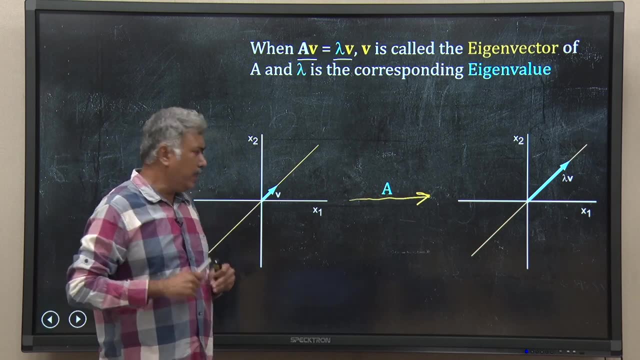 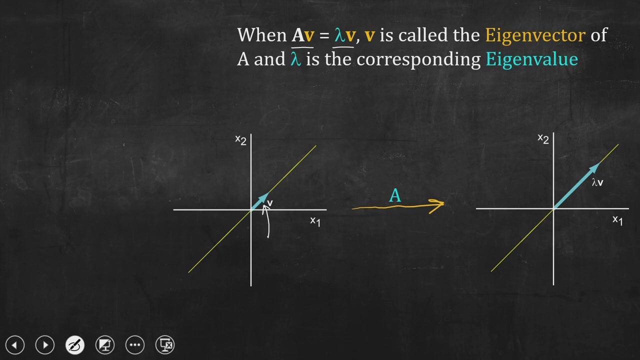 vector that will be equal to lambda into V. That is our definition of eigen value and eigen vector. What is happening? Just to remind you what we have discussed in another lecture on eigen values and eigen vectors, This is my eigen vector V. If I multiply this with A, I am doing: 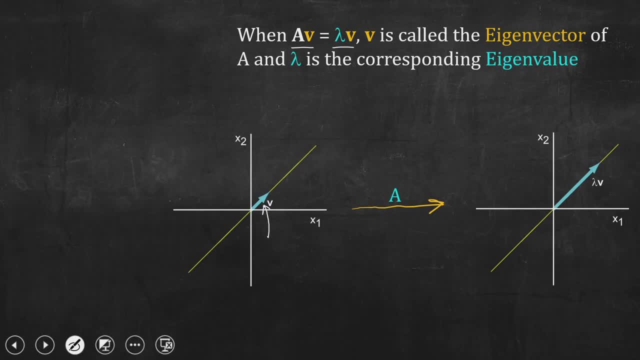 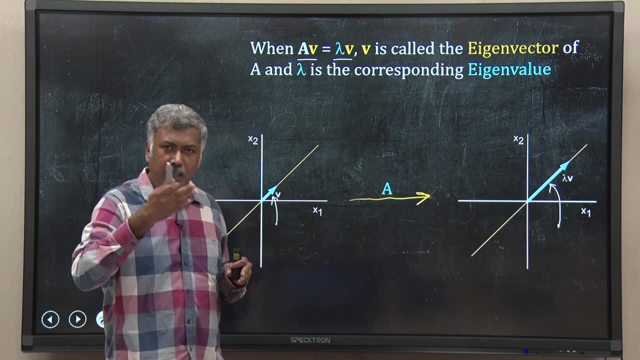 a linear transformation A into V, and then I get a new vector, lambda V. So the direction of the vector does not change, Only it remains on the same span. Either it gets squeezed, elongated or it gets flipped on the same line. That is what is called eigen value and eigen. 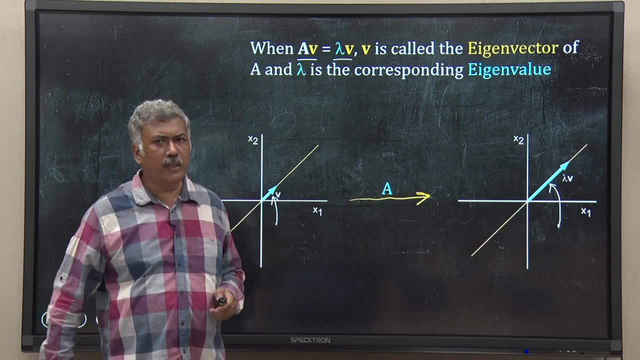 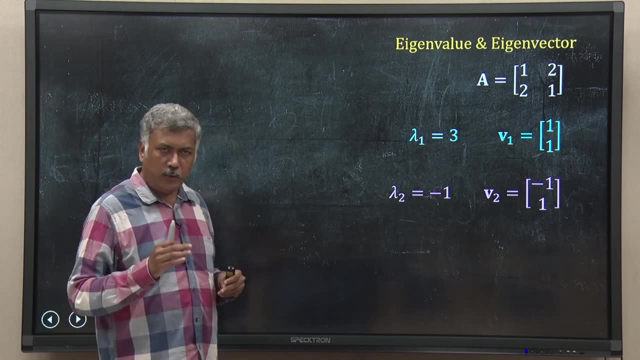 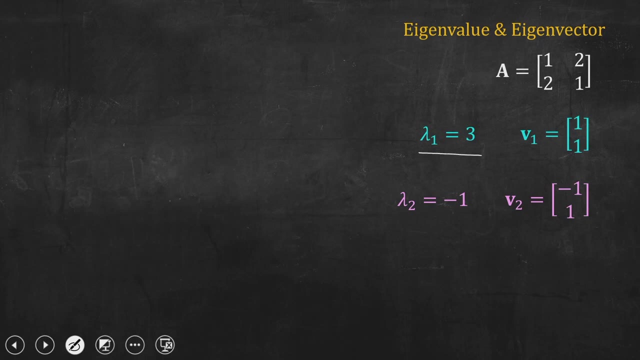 vector. So now let us take an example. We have looked into that example earlier also. So I have a matrix A- It is actually thief matrix, if you remember. So it has a two eigen 안녕 values and two eigen vectors. Eigen value 1, lambda 1 is 3 and the corresponding 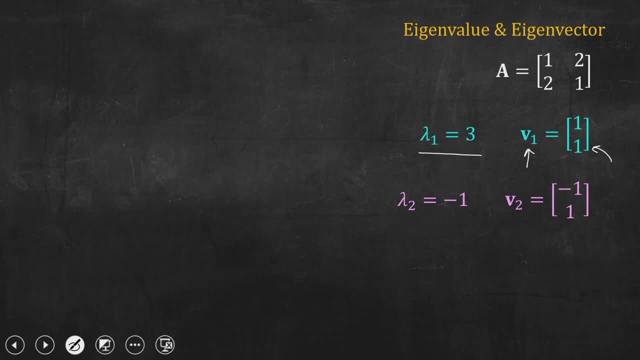 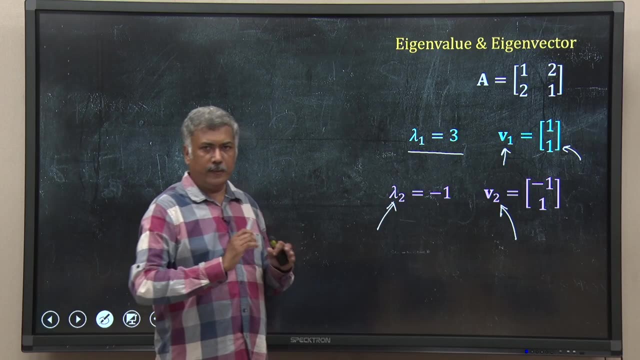 eigen vector is V1.. This is one 1, and the second Eigen value is a lambda 2 and the corresponding eigen vector is V2 minus 1.. 1& to 1%. I have colour coded them because I will mix them. 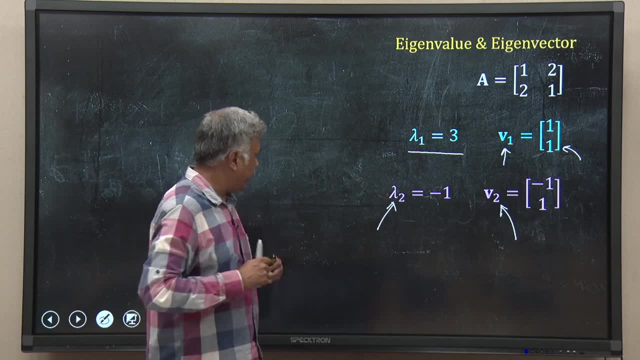 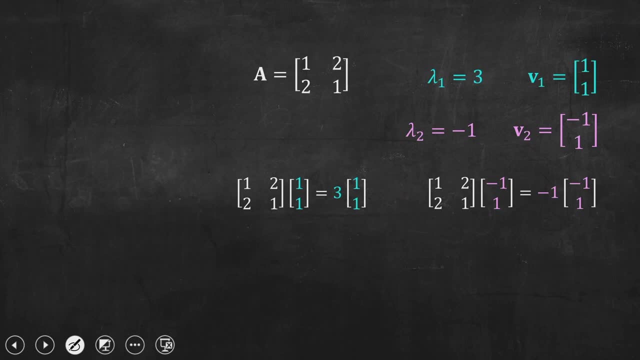 together create new matrix and vectors. so it will be easy to understand, okay. So now let me rearrange this term and write in another way. So what I have done here: I have taken matrix A and I have multiplied with the first eigenvector, V1, so I get that. 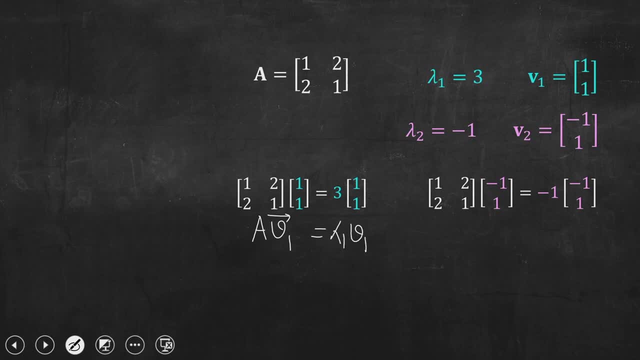 equal to lambda 1 and V1, right, That is by definition. Similarly, here I have A into V2 vector eigenvector, second one and the second eigenvalue into V2, the second eigenvector corresponding eigenvector. So I have two equations right. So I will now take this first equation. 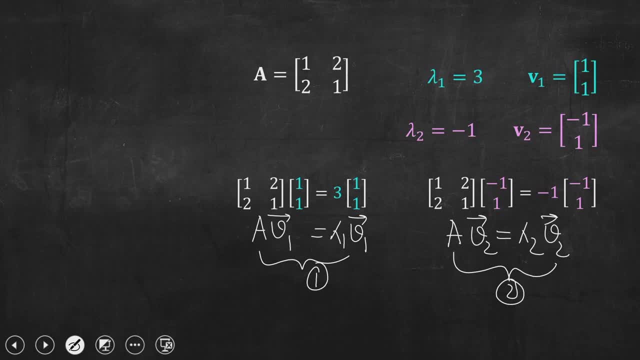 and this second equation, and I will club them together in a single unit. I will put them together in a single unit using matrix operations, right? So what I will do, Let us start What I have done. this is my A, you can see, right? I? 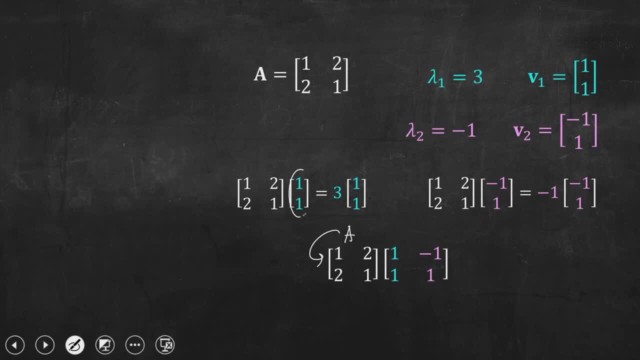 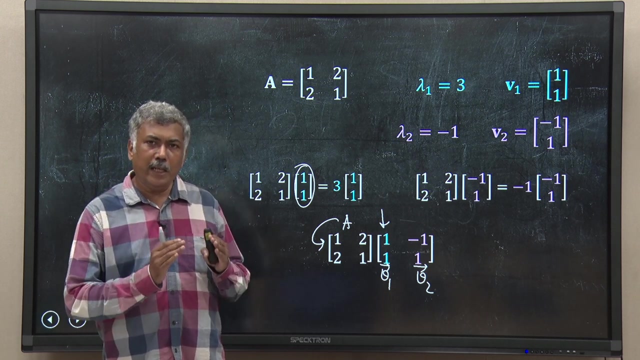 have. this is my A and I have taken the first eigenvector and put it here. So this is my V1 and side by side, arrange the V2, the second eigenvector. So I have created a new matrix using V1 and V2 and I am multiplying A with that new matrix, right? So what do I get? 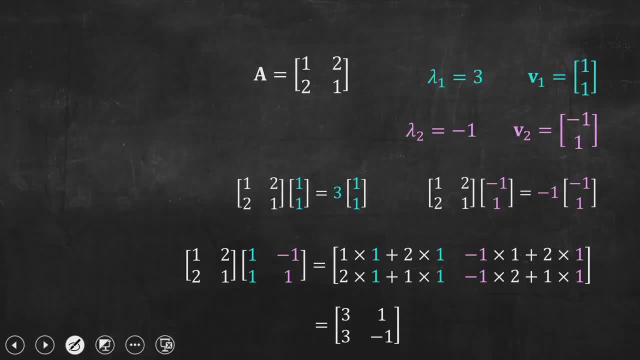 I will use the rule of multiplication of two matrices, So I get this one. You can try yourself. So first you will take this column And the first row, you will get this one. Then take the first column and the second row, So you will get this one. In this way, if you do the multiplication yourself, you will. 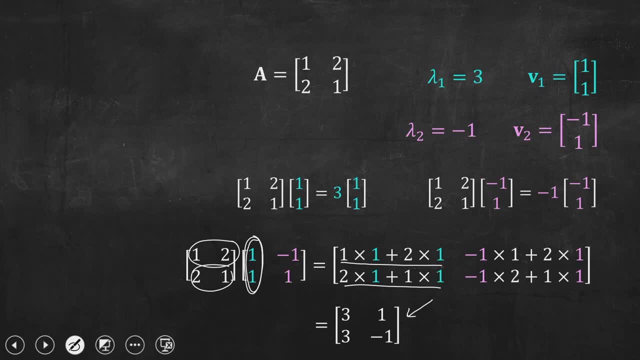 find I am getting a matrix 3-1, 3-1.. Now look carefully to this matrix. This is 3-3, right, This vector, this column vector, is 3-3.. So if I multiply my V1 vector, first eigenvector. right, My first eigenvector is 3-1 and I have just multiplied that by 3-2.. So I have D1.. V1 and D2.. So I have just multiplied that by D1.. But if I take the first eigenvector and 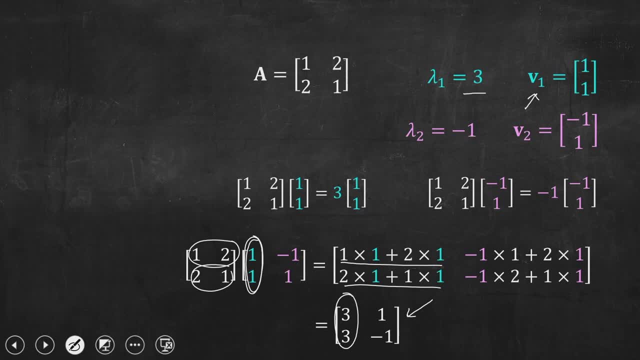 with its eigenvalue 3, I will get this vector. Similarly, look into the second column vector of this matrix that I have got by multiplication 1 minus 1.. If I multiply my eigenvector v2 by this lambda 2 eigenvalue, I should get this one. Try yourself, you will get that. 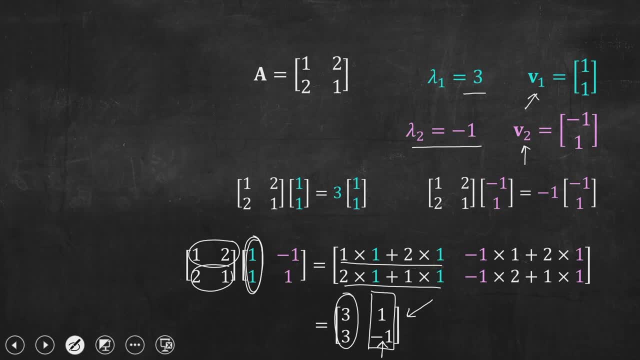 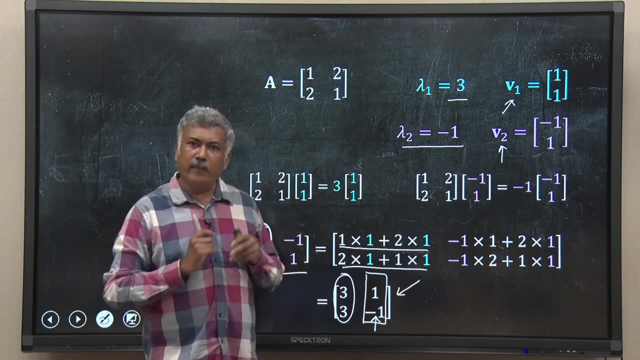 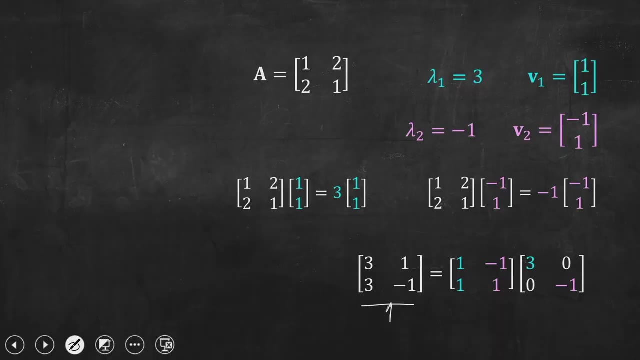 one. That means in this new matrix that I have got by multiplying this matrix, and this matrix is actually hiding those eigenvalues and eigenvectors. Let me expand that So I can write: this product that I have got just now is equal to again that same matrix. 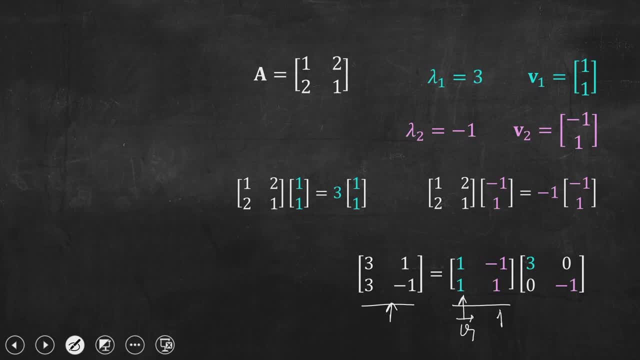 This is v1 and this is v2.. Now what I have done here in the next matrix is a diagonal matrix. Only there are nonzero elements in the diagonal of the matrix. All other values are 0.. 0.. And what are the diagonal element? The first diagonal element is this: one is lambda. 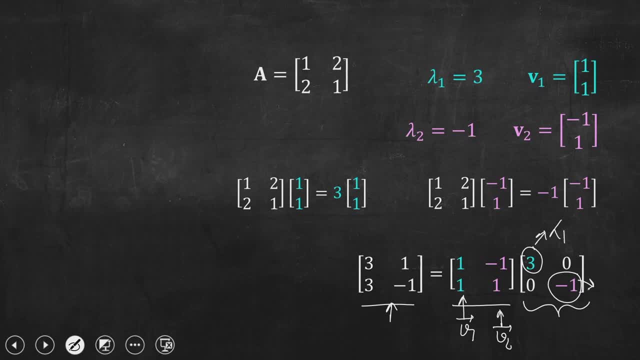 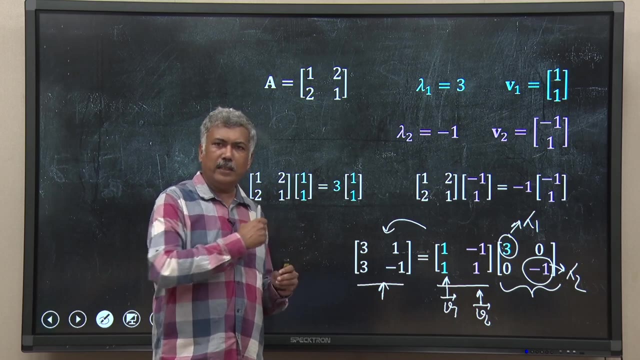 1, the first Eigen value and this one is the second Eigen value. Now you do the multiplication using the rule of multiplication of matrices, you will find you will get this matrix. So now I will equate both the thing, what I have, the multiplication that I have done. 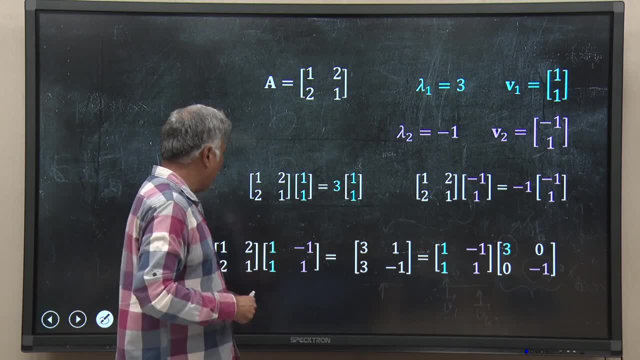 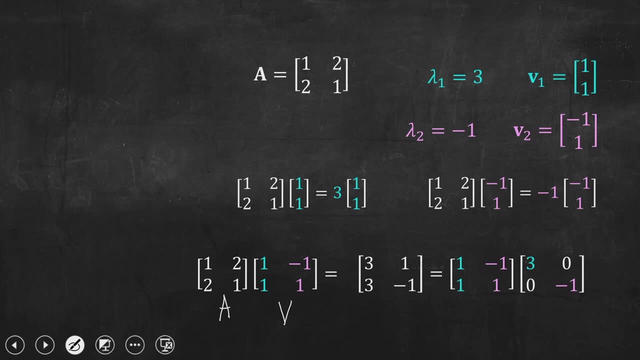 in the previous slide and the multiplication in this slide. So what I will get, I have A. I multiply that with a vector V. I will write that as a capital V because that has two column vector. The first column vector is V1, the Eigen vector, the first Eigen vector. 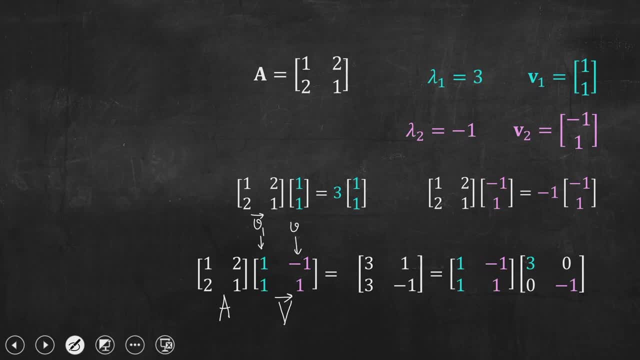 of A and it has a second column, vector V2, which is the second Eigen vector of A. that will be equal to the same vector And V matrix capital V, remember not small v- And this one I will call lambda capital. 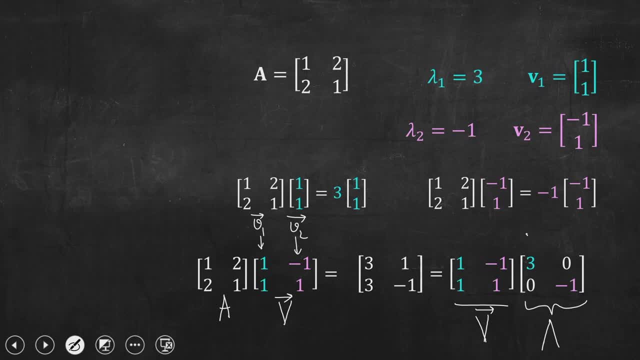 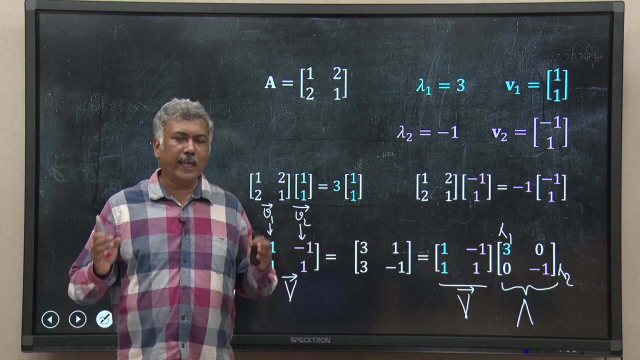 lambda because it is hiding my. it is a diagonal matrix. it is a diagonal matrix with lambda 1 here and lambda 2 here in the diagonal. So what I have got? I started with a single matrix. I know its Eigen vectors and Eigen values. 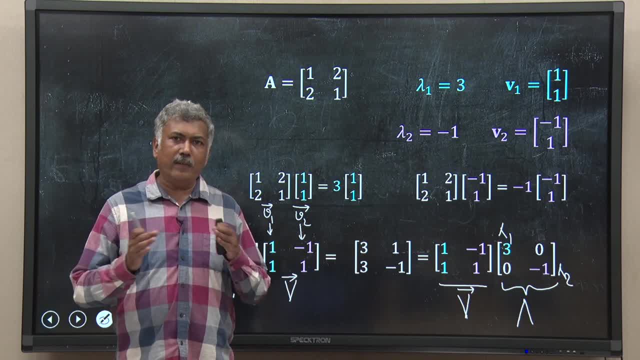 So now I have represented So what I have got. I started with a single matrix. I know its Eigen vectors and Eigen values. So now I have represented this Eigen value, Eigen vector relationship in a different way. I have written A into. 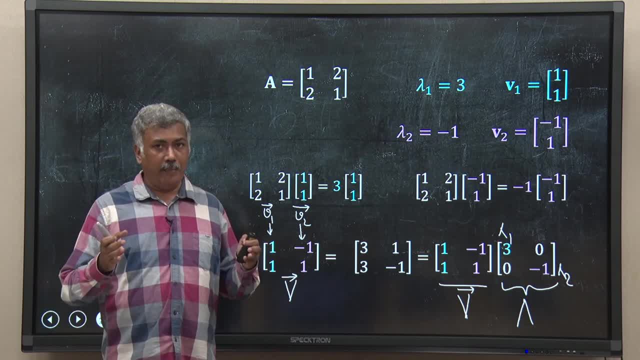 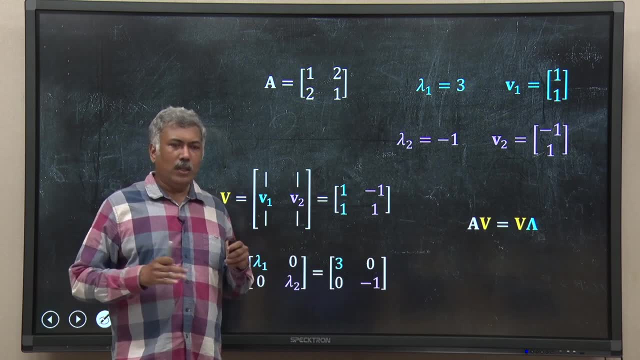 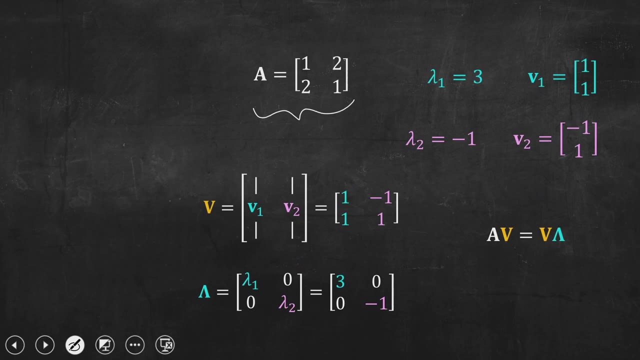 V- capital V is equal to capital V- into lambda capital. lambda Capital- lambda is a diagonal vector with the Eigen values along the diagonal. So if I just recapitulate what I have done till now, I started with A. I have clubbed the Eigen vectors to create a new matrix, V. 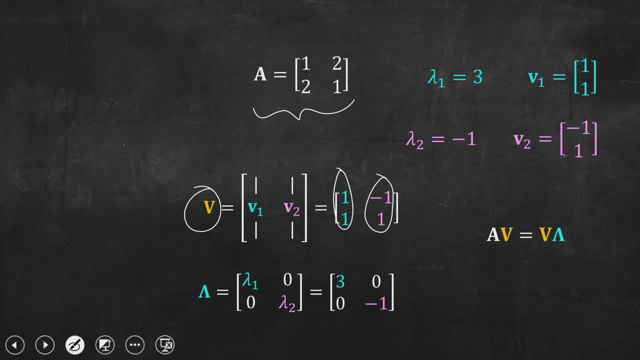 capital V, And usually in the subsequent slide I will use this symbol. This V is: this represent a column right And this is the first Eigen vector right And this represent the second Eigen vector And capital lambda. that is, a diagonal matrix having two Eigen values. 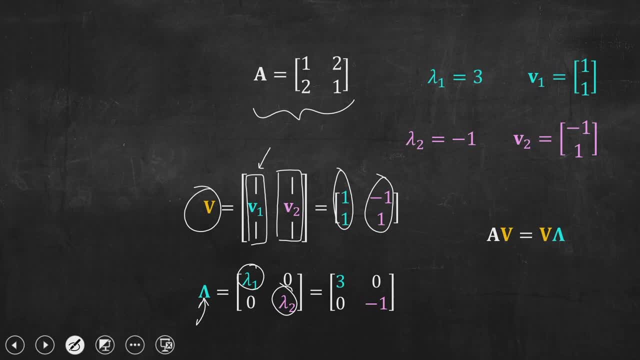 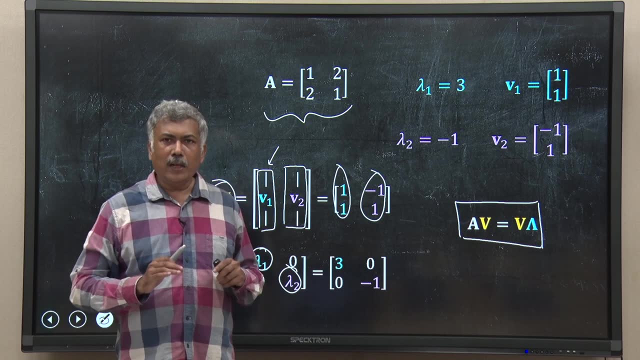 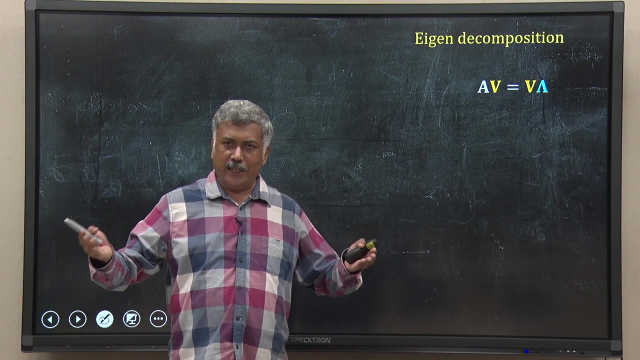 along the diagonal, And that gives me a relation that A into V is equal to V into lambda. So now comes the part of Eigen decomposition. What is the meaning of decomposition? You want to break down something into parts, right Components. So that is what we want to do. 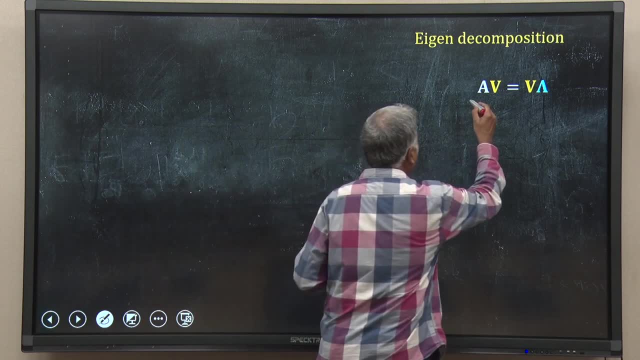 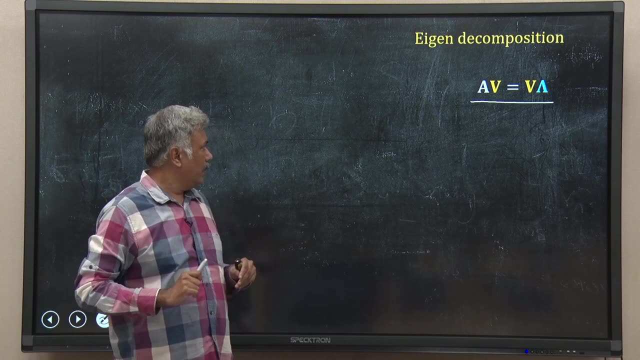 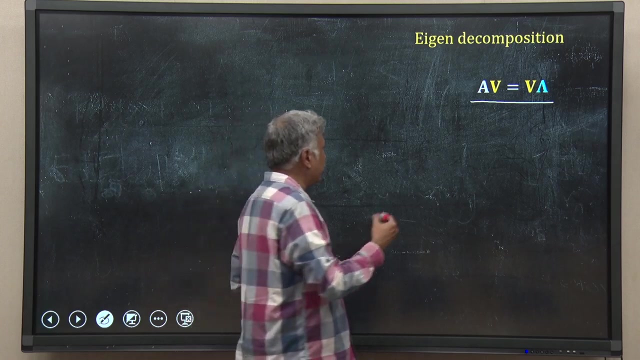 in Eigen decomposition I have proved the relationship A into V is equal to V into lambda. I hope you remember what is V capital V and capital lambda are. Now I want to separate out A from this relationship. To separate out A, the simplest one would be. 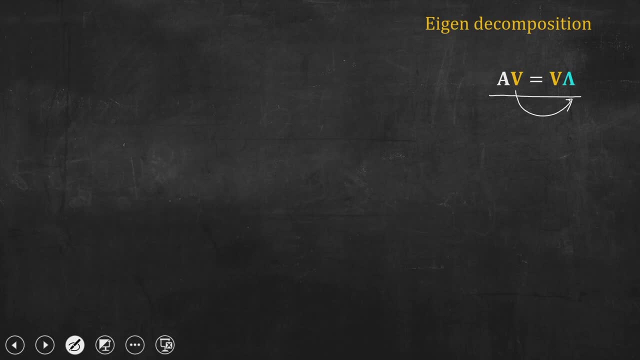 if I can take on this side the V on this side. but I cannot do division by a matrix right. But I can do inversion. So what I will do, I will multiply both side by V inverse right. So if I multiply I will get A into V, into V inverse equal to V, into lambda, into. 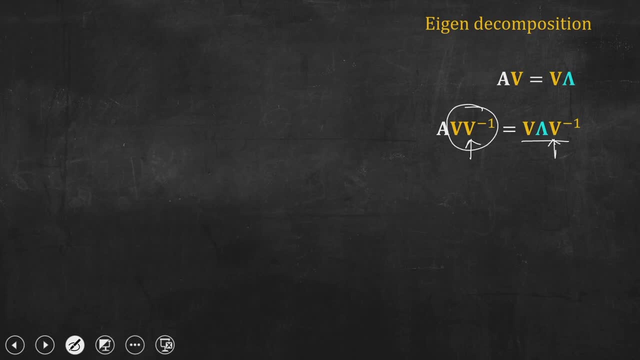 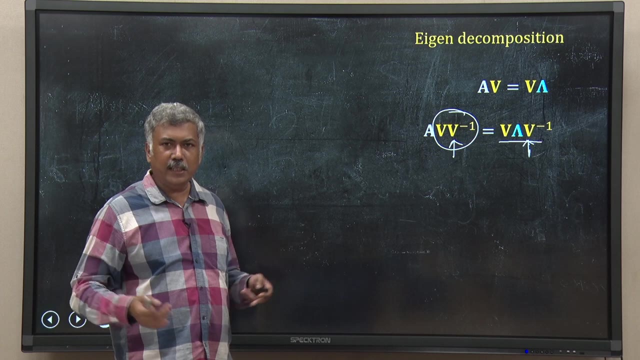 V, inverse. Now, what is this? This is the identity matrix, right? If I multiply this matrix, which is inverse, I should get an identity matrix by definition, and identity matrix is equivalent to 1.. And if I multiply a matrix with identity matrix, I will get: 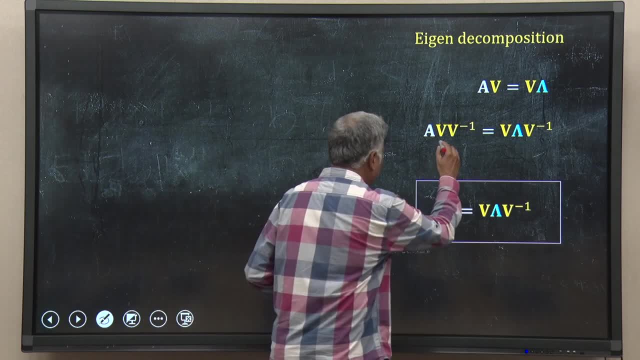 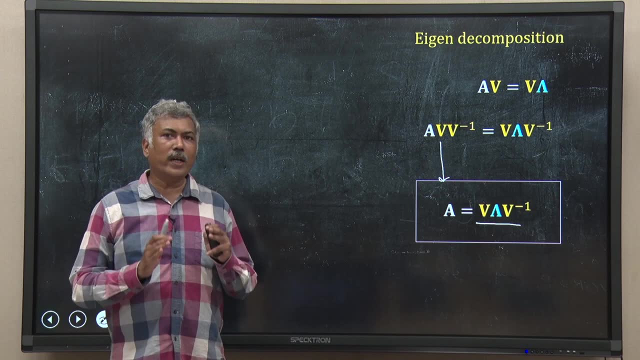 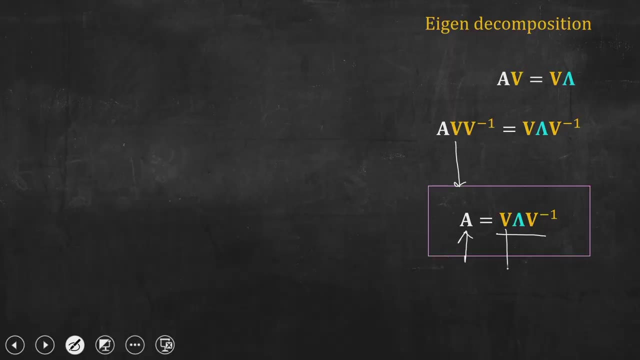 back the same matrix. So I will get A equal to V into lambda, into V, inverse. So what I have done, I have broken down, I have decomposed the matrix A in three parts, right, And what are those three parts? Let us look into it. So this is my square matrix n into 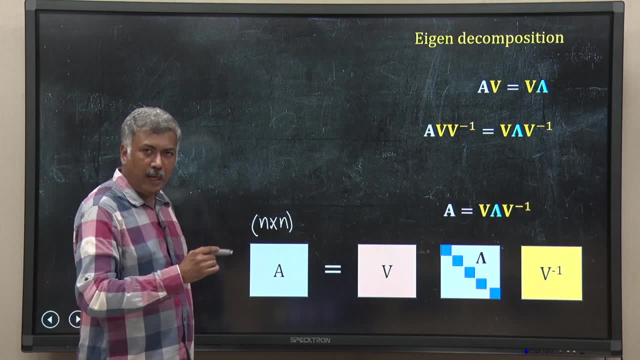 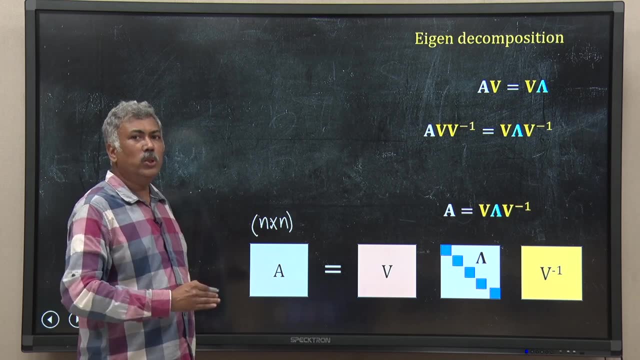 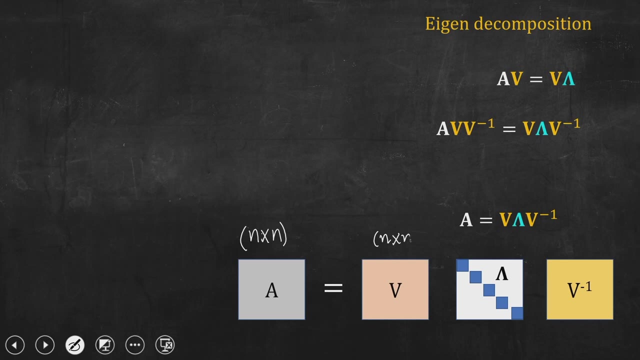 n. Just to remind you again, because we are using eigenvalue eigenvectors, so we have to deal with square matrix. So I have a square matrix A given to me. I have broken it down into three components, right, The first is also a n into n, where I have all the eigenvectors. 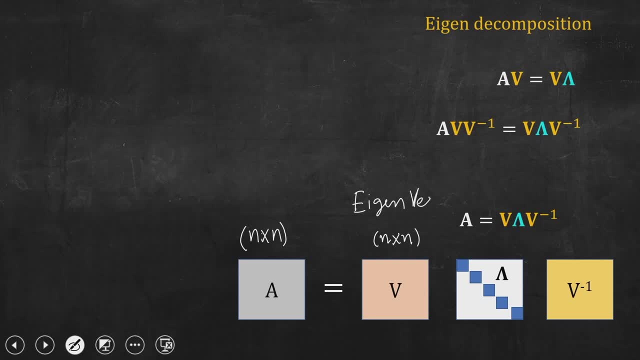 I have the eigenvectors stacked side by side right, And then I have n into n diagonal matrix. That is why I have used this type of color in the diagonal. I have a diagonal matrix where I have all the eigenvalues, corresponding eigenvalues. right I have quatre-formation valleigichts. 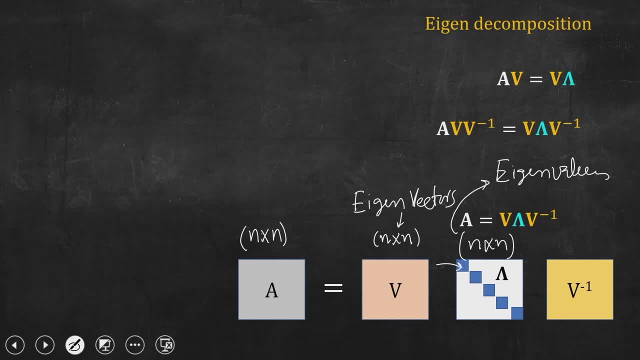 dragged hatch-edstonius-had direction- Whavelthatting-and-theretelementade. competitors are different. There are different halves. I have hn over h by Krebelää, I have U over V times the diagonal. So they are. 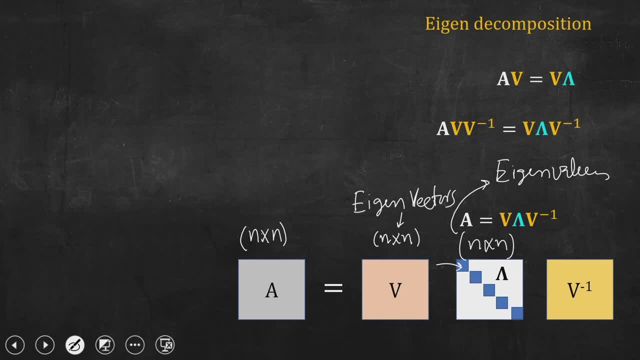 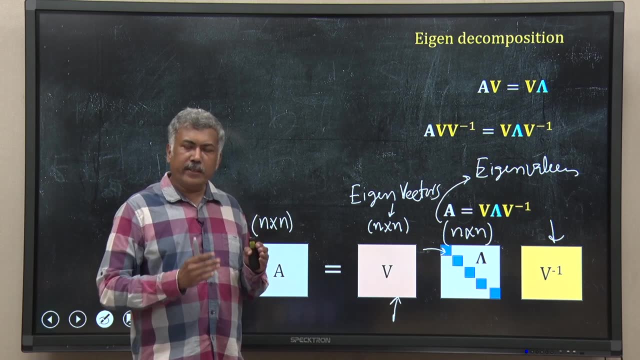 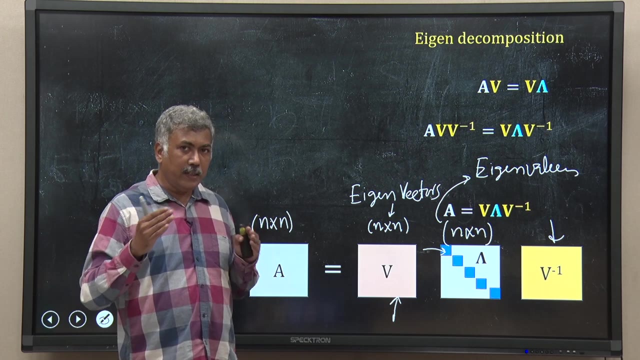 diagrams. I have h1 over V. I am going to write out a ultimate matrix that I will show little by little. So in the diagonal, and this is the inverse of the first matrix, V, that is also a square matrix. So one square matrix is now divided or decomposed into three square matrices. And remember one thing: 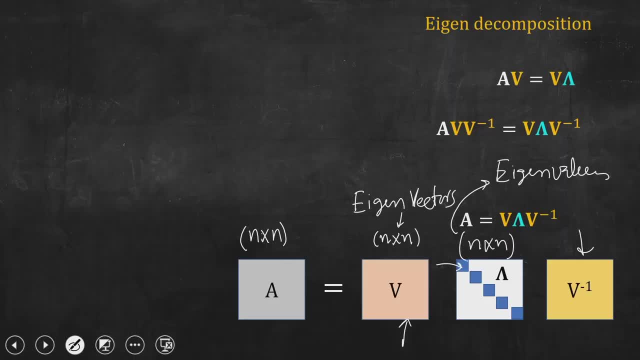 we do usually in data analysis. what we do? we arrange these eigenvalues in order. that means the first eigenvalue at the top most corner will have the highest value, then the next one, then the next one. So that means the eigenvectors are also arranged correspondingly. So this is the 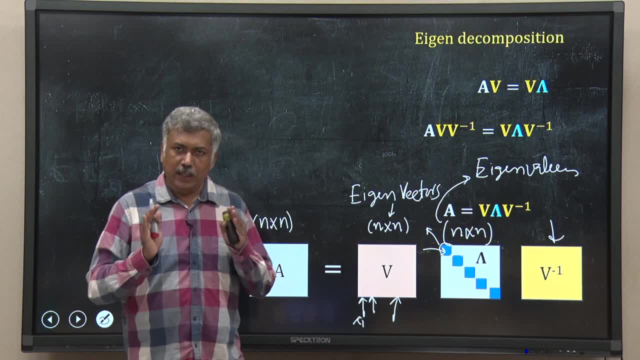 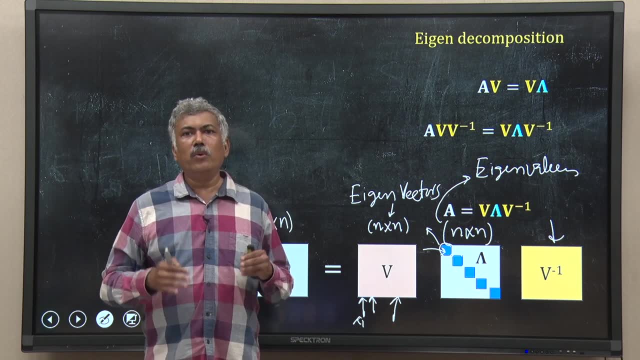 highest eigenvalues, eigenvector in the first column, something like that. We do that because in data analysis sometime what we do, in particular some dimension reduction techniques, what we do, we only consider those eigenvectors and eigenvalues which are more important, that means their values. 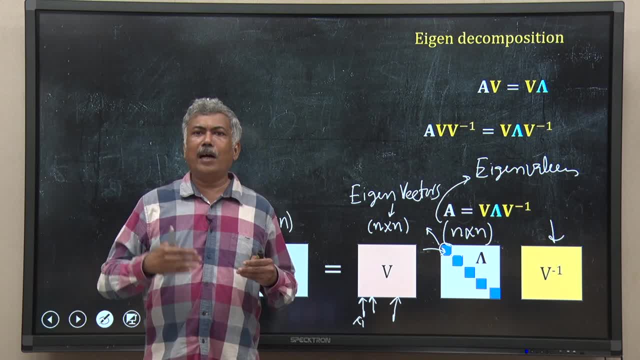 are higher, eigenvalue values are higher, So we may discard eigenvalues and their corresponding eigenvectors when the eigenvalues are very low. So that means we do that because in data analysis sometimes what we do, in particular some dimension reduction techniques, what we do in particular, some dimension reduction techniques, what we do in particular, 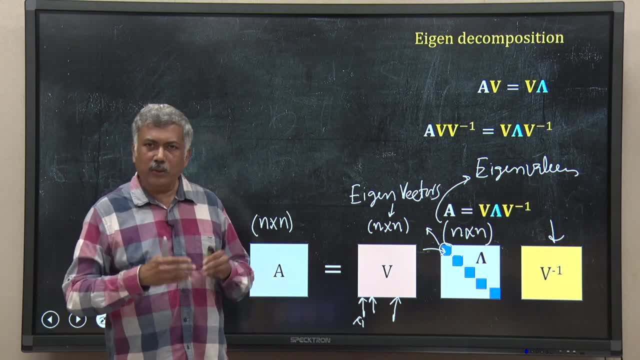 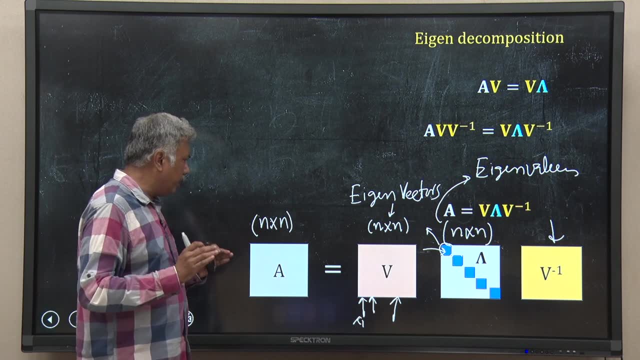 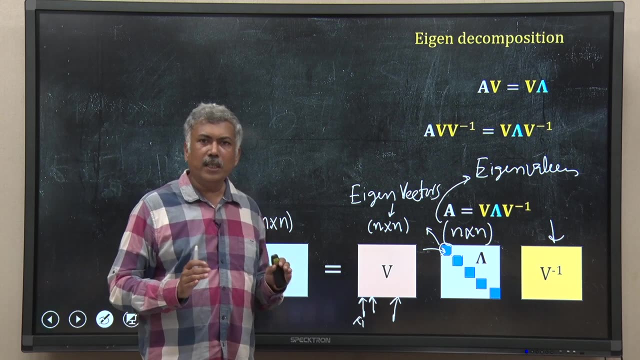 so if you arrange them in order, then it must become easier to implement. So that is why you arrange them in that particular order. So just briefly repeat. let me repeat what we have done. we started with a square, matrix A, and we have decomposed it by eigen decomposition into three. 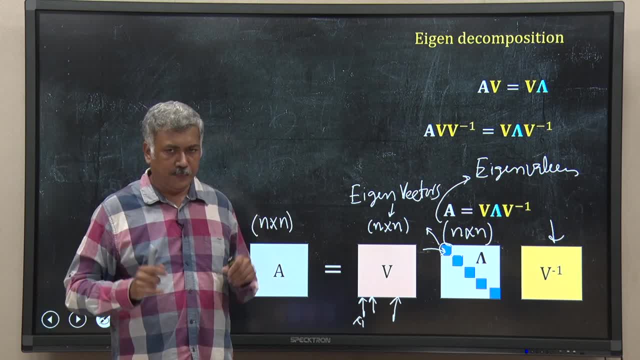 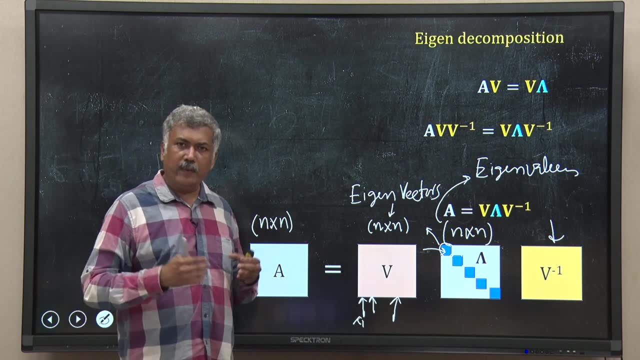 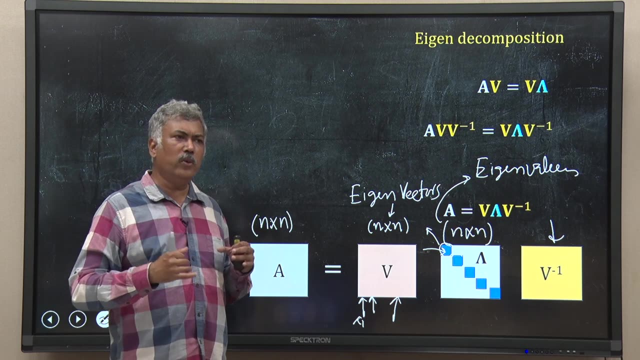 parts right, V into lambda, into V, inverse, And this method is very useful. you may think why we are doing all this juggling of matrices, vectors and eigenvalues. eigenvectors Because this is very useful technique, because under the hood, many algorithms, for example you. 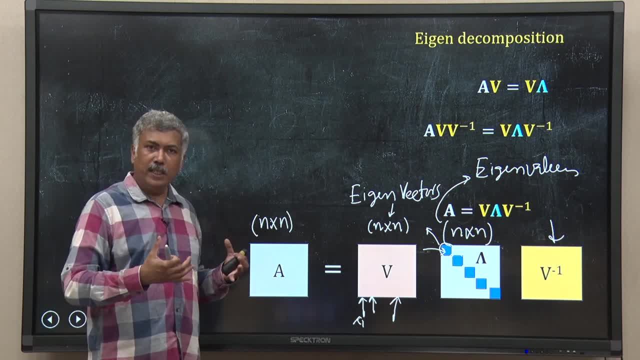 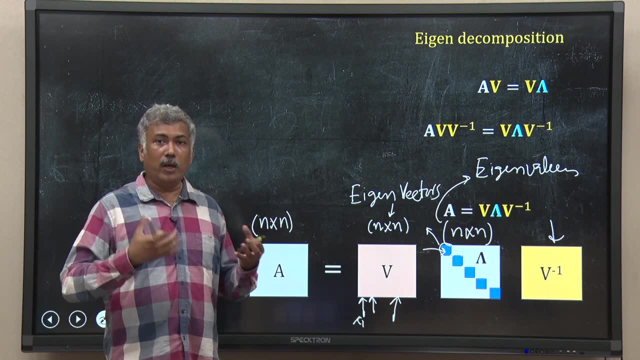 have to square this matrix or cube this matrix, Is it very? not a trivial job to do. but if you use eigen decomposition and then try to calculate the cube, or square, or higher order of A, it becomes very easy. It becomes easy because you have to remember we 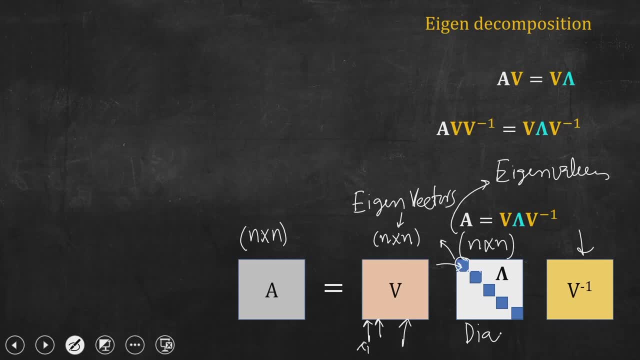 have a diagonal matrix here and the mathematics of diagonal matrix And the matrix becomes much easier to calculate. But it is not easy because you have to remember we have a diagonal matrix here And the mathematics of diagonal matrix. it is not so easy. you have to understand. it is not possible to print out. 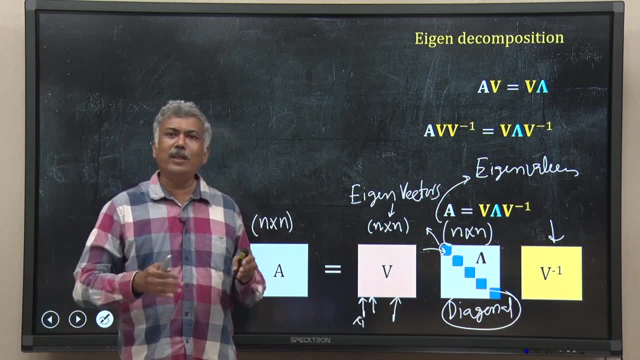 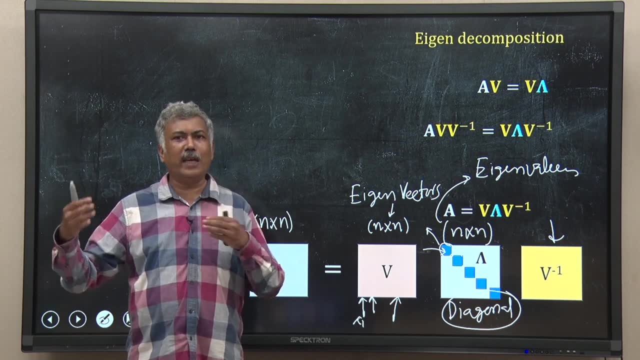 matrix of diagonal matrix is very easy because it had only non-zero element in the diagonal. All other elements are 0. So most of the multiplication, addition, all this thing gives rise to 0 and it is a square matrix in this case. So it transpose is also a diagonal. 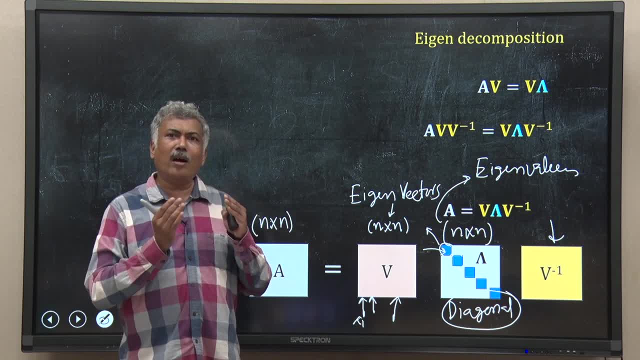 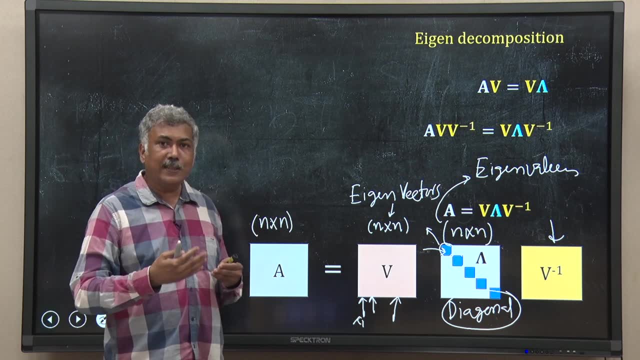 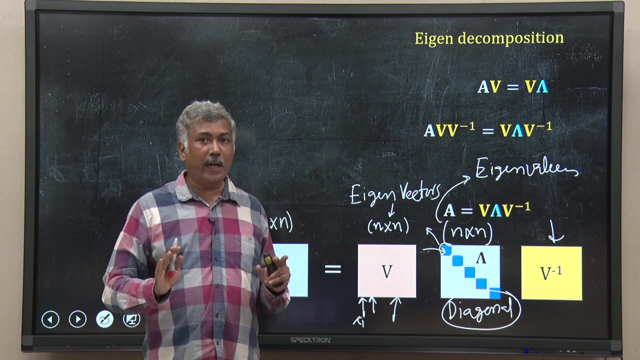 matrix. So as the math of diagonal matrix is very easy, as we decompose the matrix in A in this fashion, the further analysis of A also becomes very easy. So far, so good. I have decomposed a square matrix A, But the problem is in most of the data analysis that 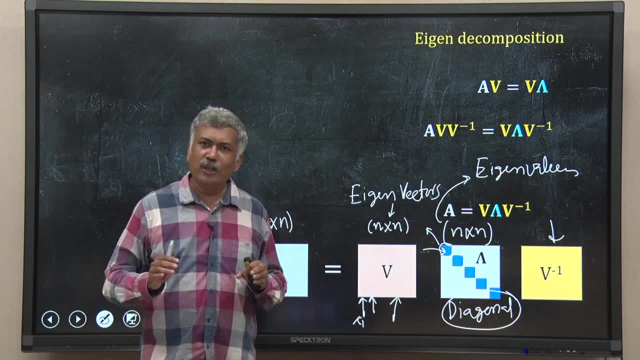 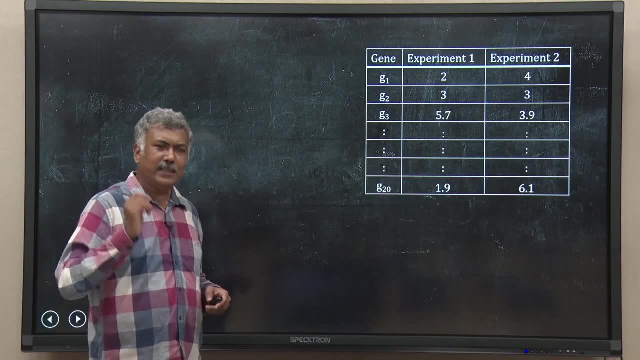 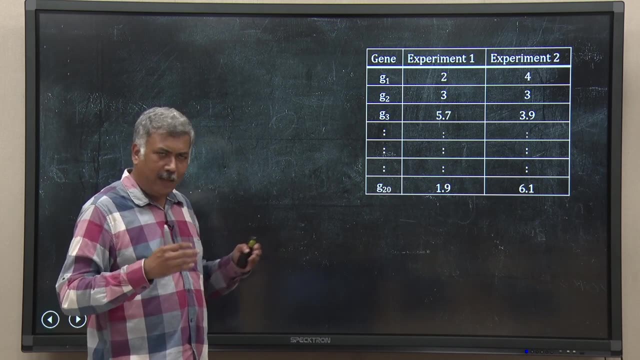 we will deal in real life, particularly in biology. also, most of the data will not give you a square matrix, It will give usually rectangular matrix. Just remind you, let us see one data set that we have handle earlier to understand matrix and vectors. So this is a gene expression experiment data, a hypothetical one. So I have done. 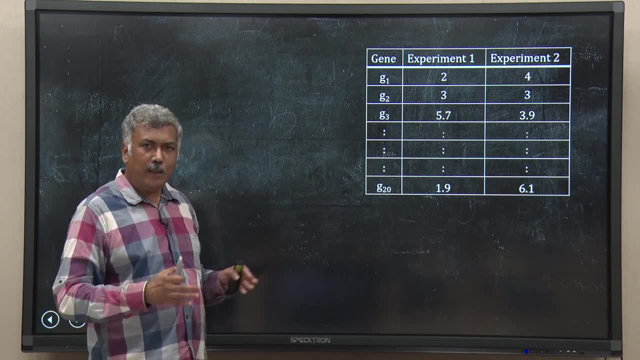 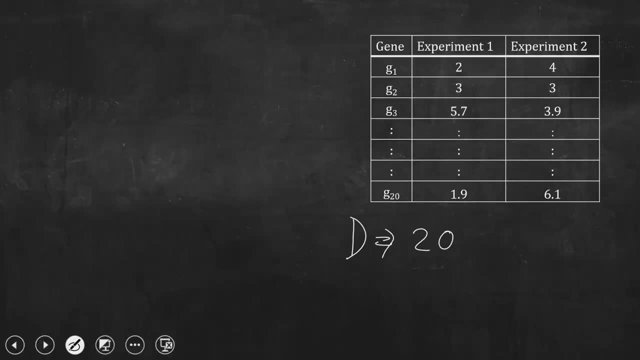 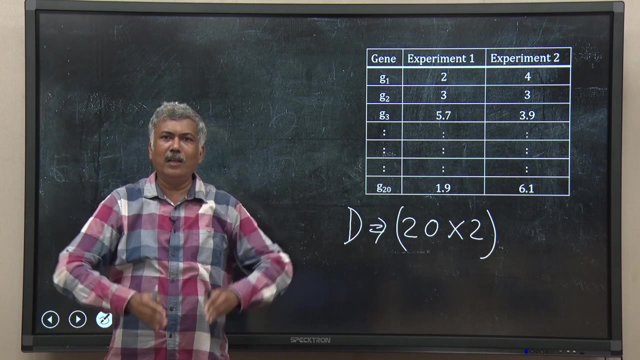 two experiments and I have 20 genes. So if I represent these as a matrix, my data D matrix will have the dimension of 20 rows into 2 columns. So it is no square, It is rectangular, It is skinny, tall matrix And in reality if you do a microarray or RNA-seq analysis in 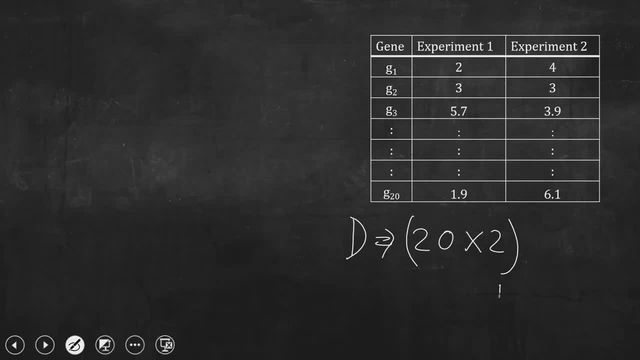 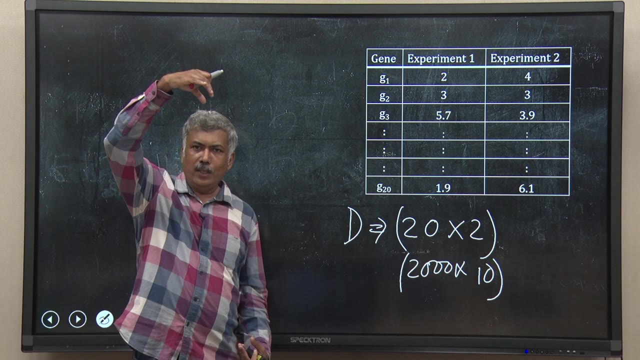 that case maybe your experiments will be a 10 at max, because these experiments are very costly to do. So you may have 10 experiments and you may have 2000 genes. So you can imagine these are tall, skinny matrices, rectangular. You can have the opposite one also in some experimental. 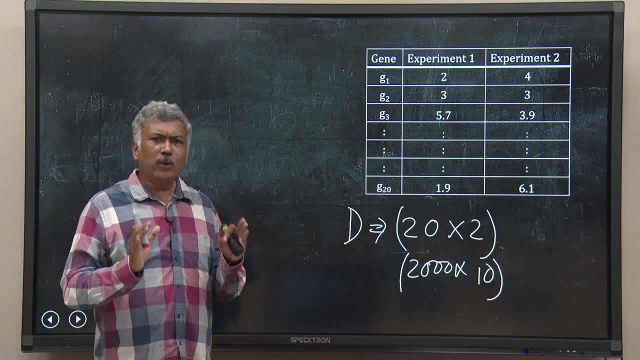 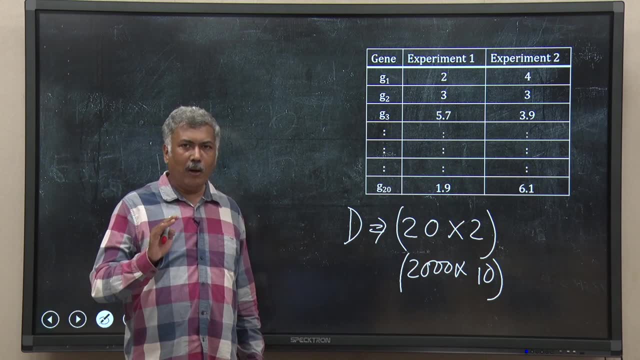 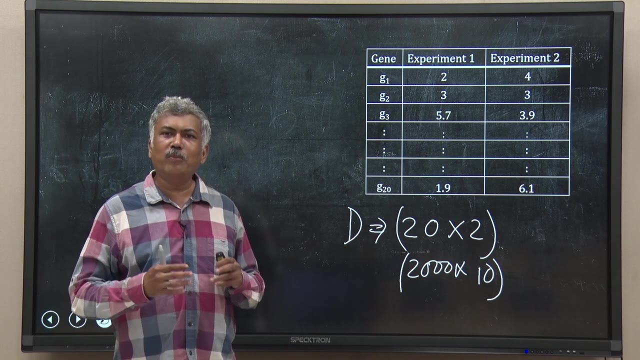 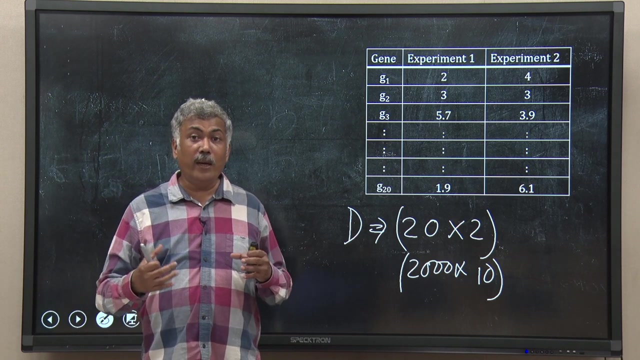 cases, some particular data set. But whatever it is, in most real life cases, particularly in biology, that data analysis that we will do. you will not have square matrix, You will always have. 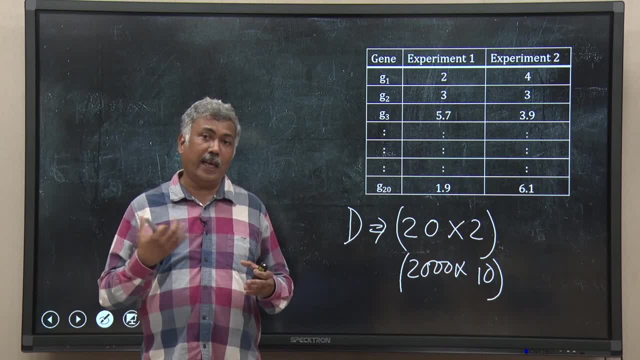 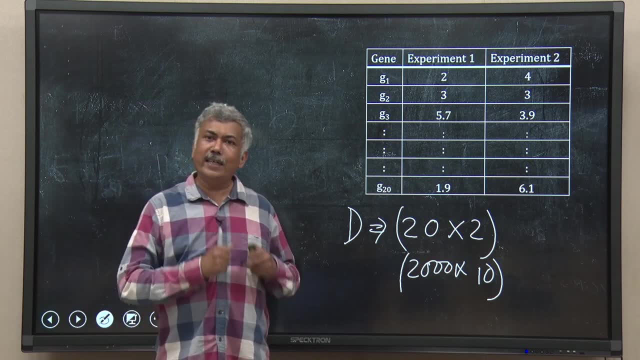 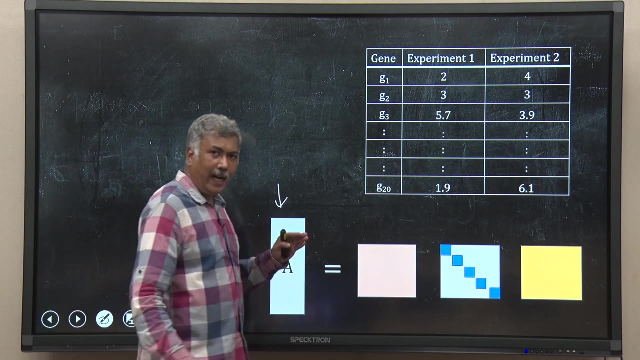 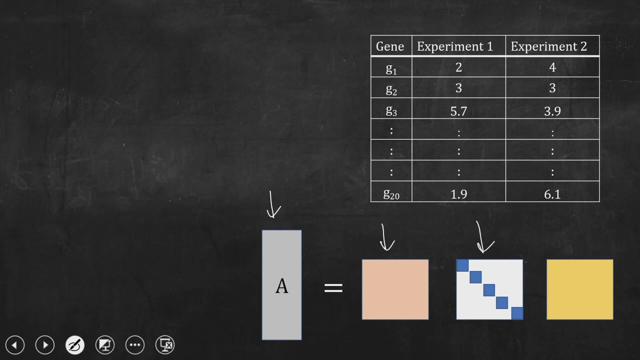 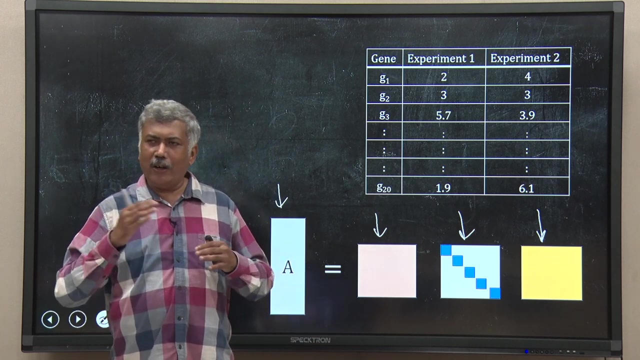 matrix And I want to decompose in a three part: a square matrix, a diagonal matrix and another square matrix. that is all. Remember if I can bring down my data or something to. 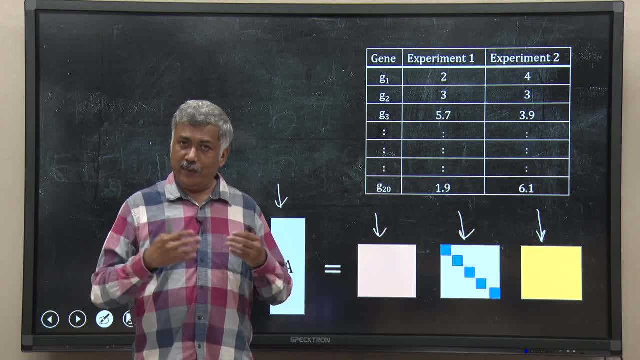 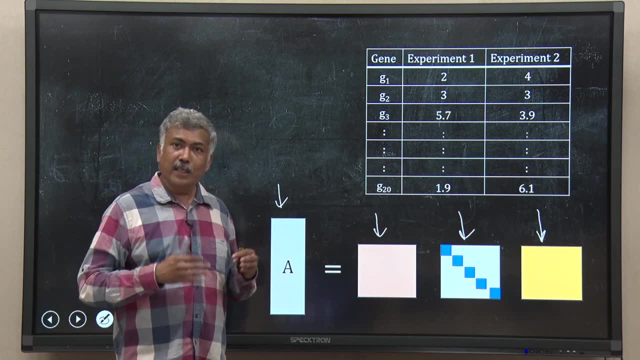 square matrix. math is much and well known, well established, very easy. lots of tools are there. If I can create a diagonal matrix also, lots of info tools are there and math is easy. So I want to decompose my rectangular matrix in this way, And that is where singular. 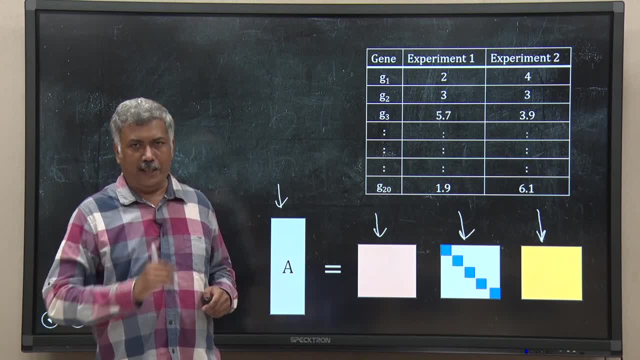 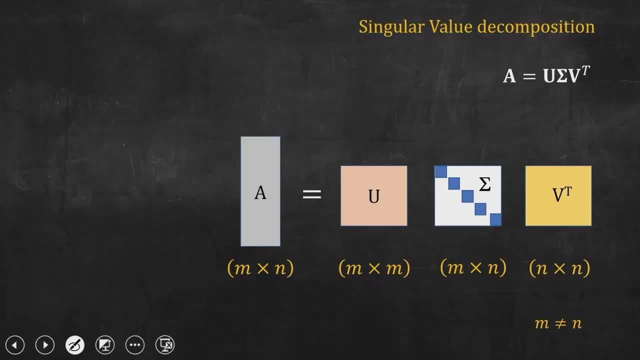 value decomposition. SVD comes. Let us learn that. So what is SVD? SVD will fulfil my wish. The wish is: I have a square matrix A of dimension m into n where m is not equal to n. in general, For this particular drawing I have shown. 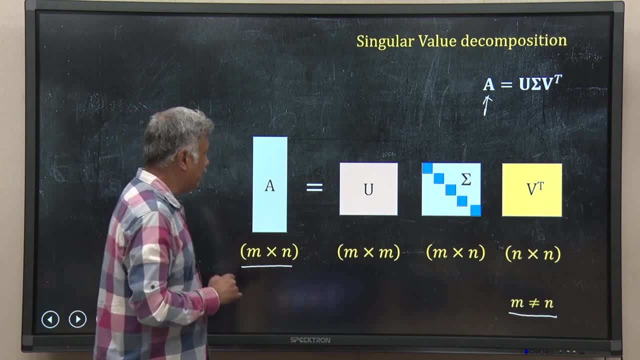 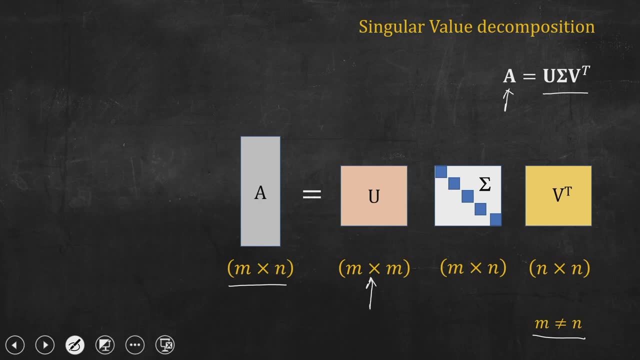 m is bigger than n, Number of rows is more than number of columns And I will break it into three components. U will be a square matrix of m into m, V transpose. the last component will be a n into n square matrix And I will have a diagonal matrix here in the middle whose dimension will be: 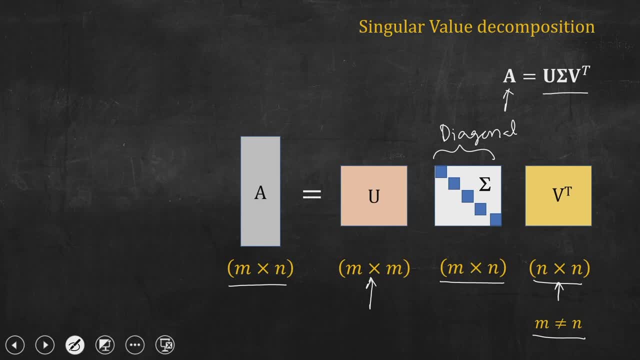 m into n, Just like that. Okay, Okay, Okay, Okay, Okay, Okay. So let us try to use the rule of multiplication. This is m into n, This is m into m, So m in m matching, whereas this n and n are matching. So eventually I will get a matrix by multiplying. 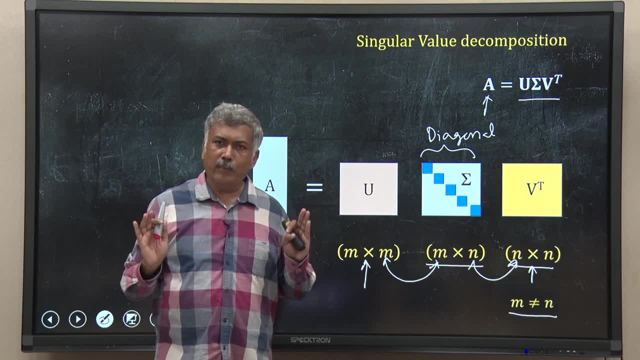 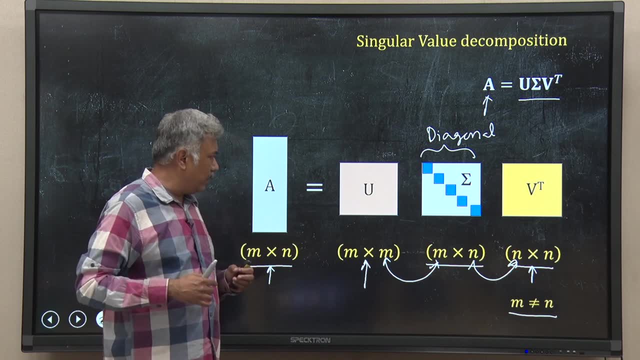 these three matrices, m, into n matrix. So the rule of multiplication is satisfied. So this is what I want, And as I want it. just this wish will not fulfil my wish. So what I do? I have to put some more constraint in it, And let me describe it. So let me. 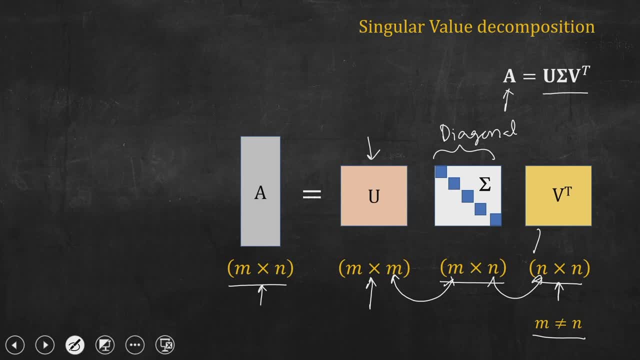 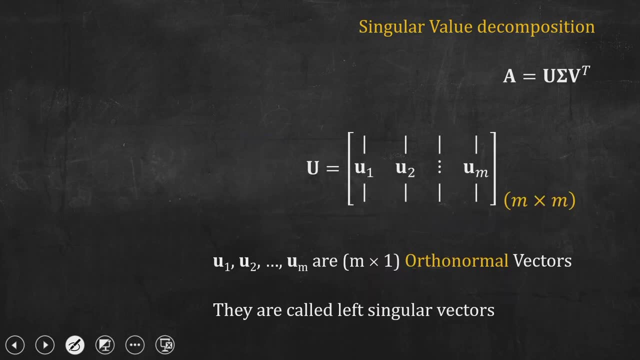 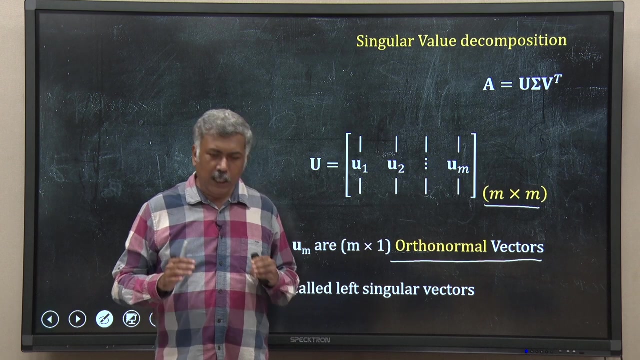 discuss what will be the form of U and V and this sigma right which is the diagonal matrix. So the U, I want the U, should be a special type of square matrix. It is obviously m into m, but it is a square matrix of orthonormal vectors. Now, what is orthonormal, If you? 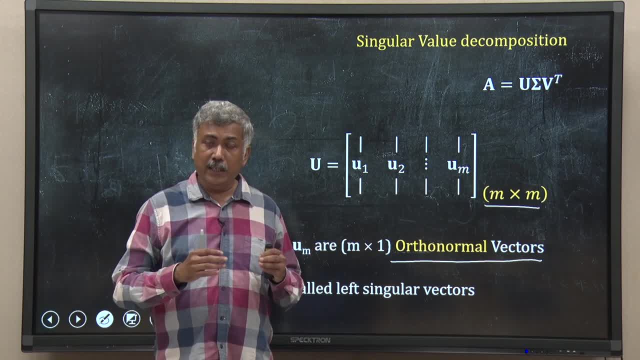 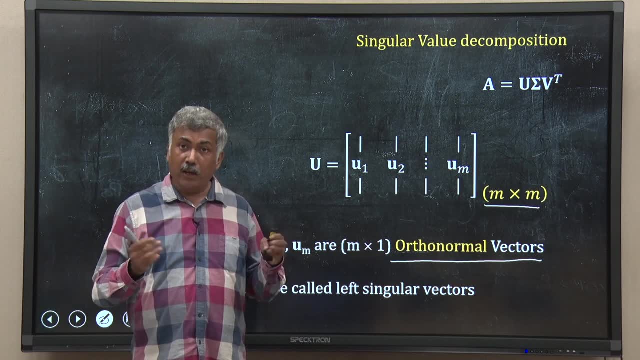 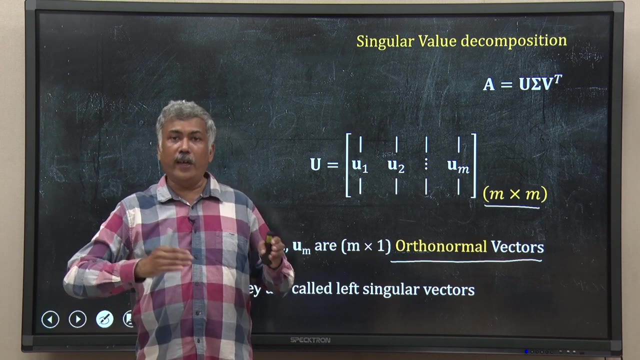 remember the lecture of vectors. we started the linear algebra discussion with vectors. right In that case I have discussed that two vectors are orthogonal or perpendicular in layman terms, if that dot product is 0, right Now, if both the vectors are unit, vector means. 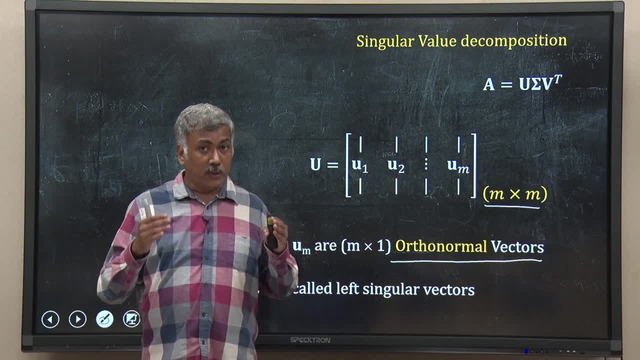 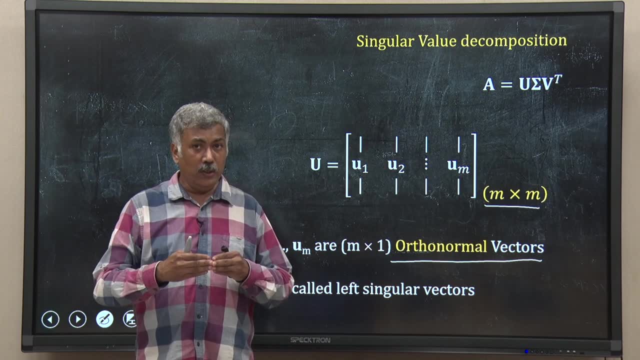 you have normalised with respect to their individual length. So if I have two unit vector and they are orthogonal- that means they are dot. product between them is 0, then we call them orthonormal right Orthogonal normalised vector- Orthogonal. you have to. 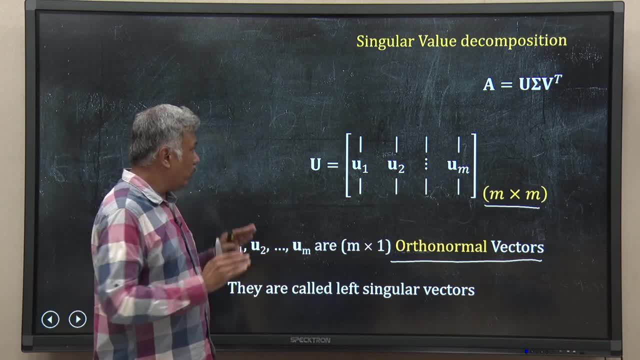 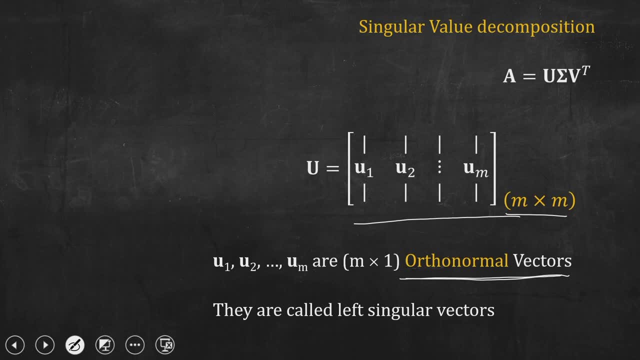 are one unit vectors, So that is called orthonormal vectors. So what I am assuming here is that this U is a square matrix having orthonormal vectors, So all these vectors are unit vectors and they are orthogonal to each other, right? 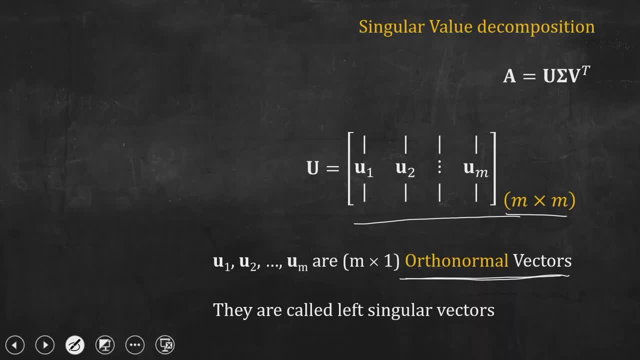 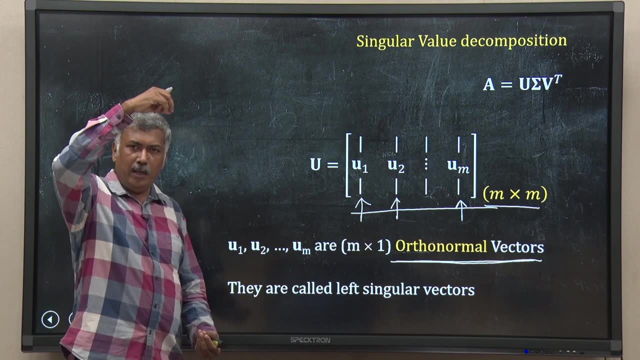 So U 1,, U 2, U m and I represent them by these notation. This is one vector, this is another vector. up to I have m number of vector and their length is also m. they have m rows right. So I have a m into 1 size vector, M number of vectors And what is m There is. 1 number of vectors, right? So if I have m and 3 vectors, then what I do is I have m into m, So they are orthogonal to each other. Okay, So with that there is a sense that if I have, 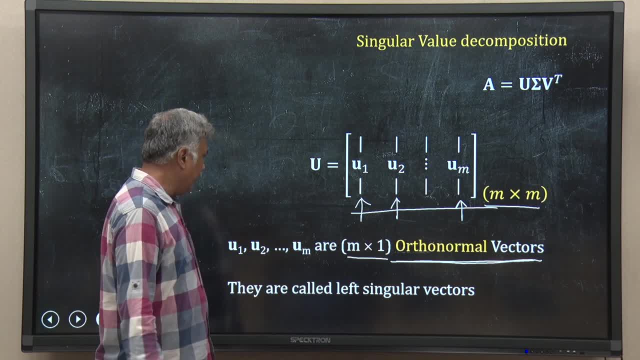 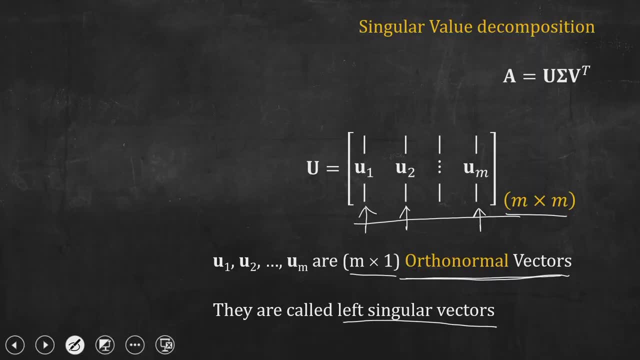 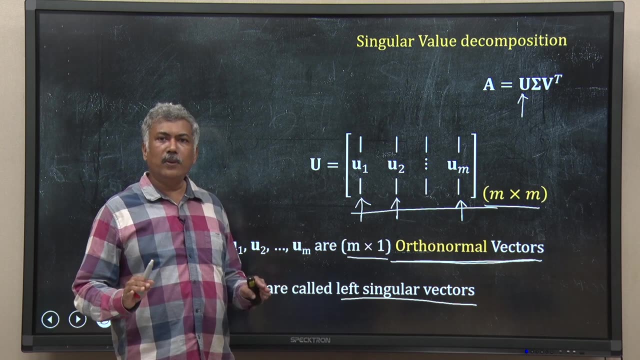 vector m, number of m, into one size vector. and these vectors? let me tell it at the very beginning: these vectors will be called left singular vectors because they are on the left side of this equation. right, they will be called left singular vectors and they are orthonormal. 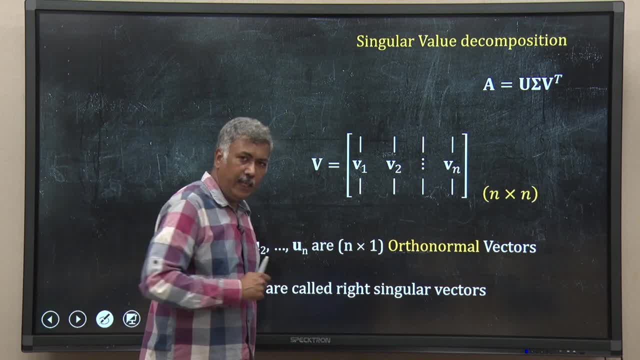 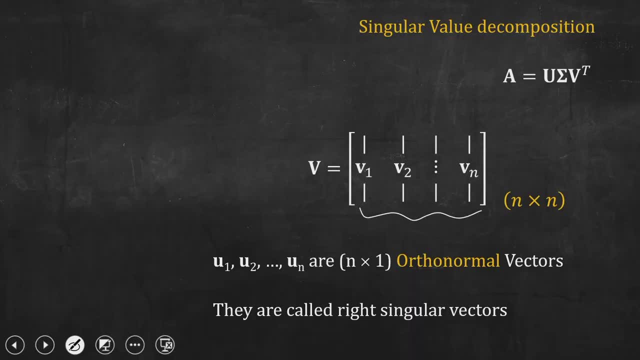 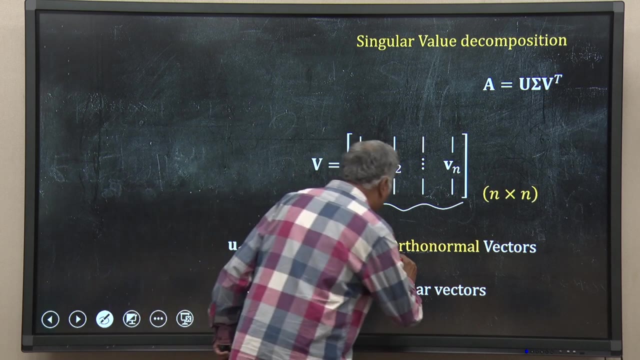 v is also similar. although you are writing v transpose, i am defining v here. v will be a n into n matrix, where it is made up of vectors, n number of vector. each of them has n into one size right n rows, one column right vector, and they are also orthonormal. that means these: 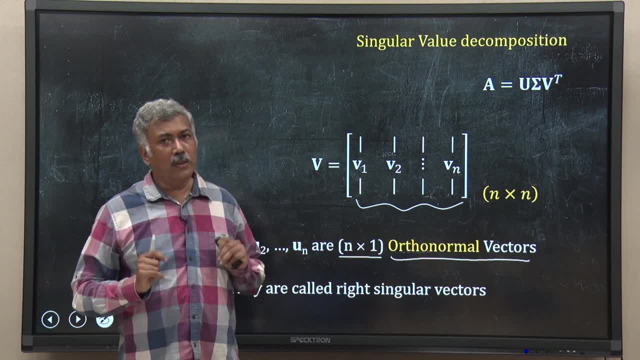 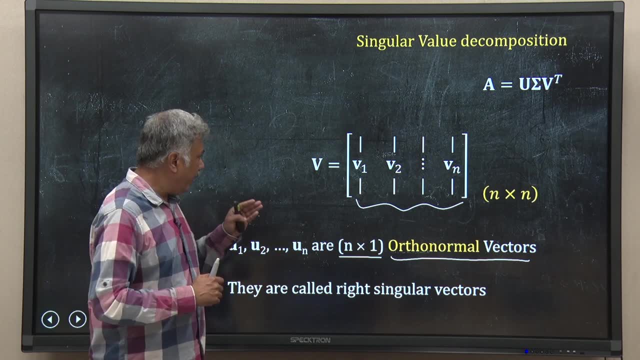 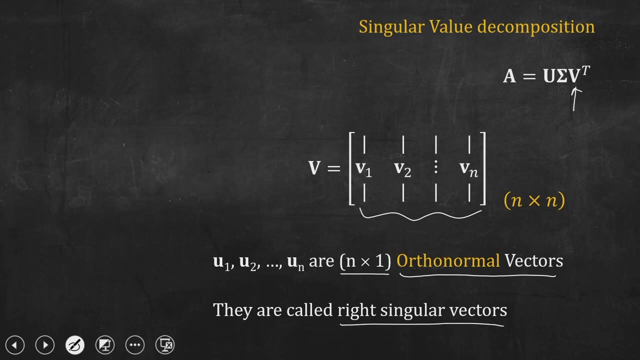 vectors are unit vector and they are orthogonal to each other. so this is the condition, same as that for the u matrix, and the vectors here will be called right singular vector because, okay, right singular vector v is on the right side of sigma right. that is why we will call it right singular vectors. 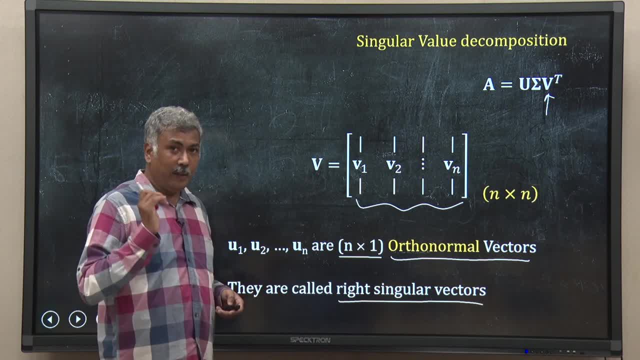 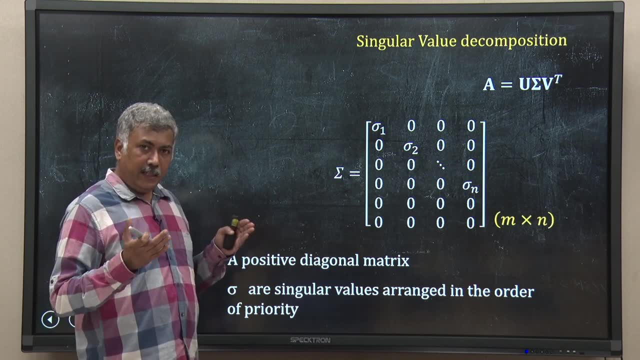 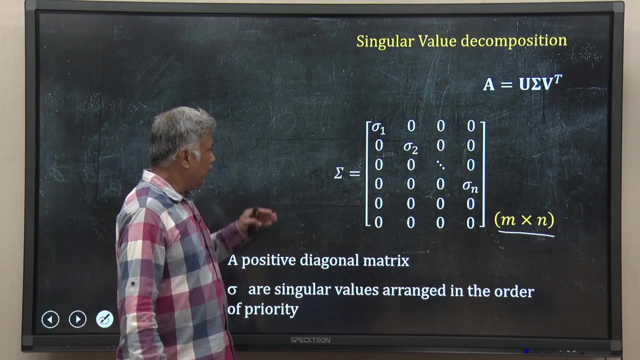 not so difficult to remember. now come the middle part, which is the diagonal matrix right. so in sigma capital sigma is a rectangular matrix because i have to match the dimension in multiplication right. so m into n. in is a diagonal matrix, so it is diagonal, has some term which are non-zero. i will call them sigma 1.. 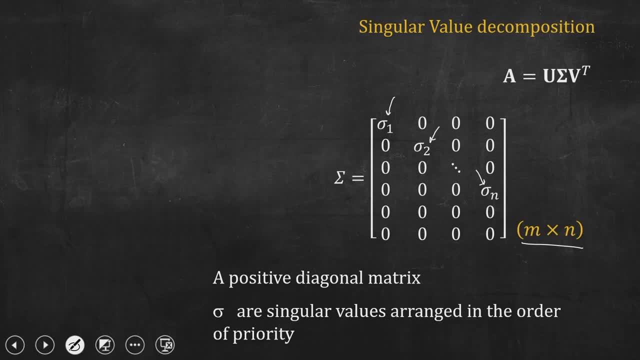 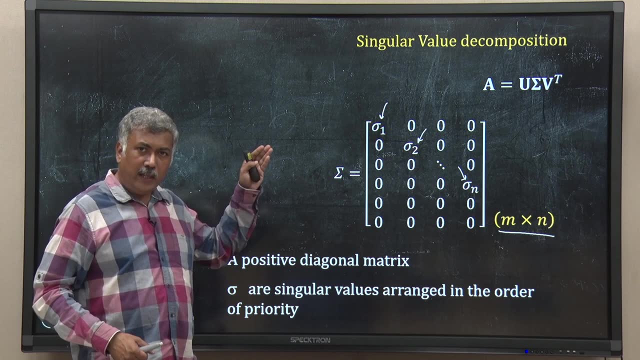 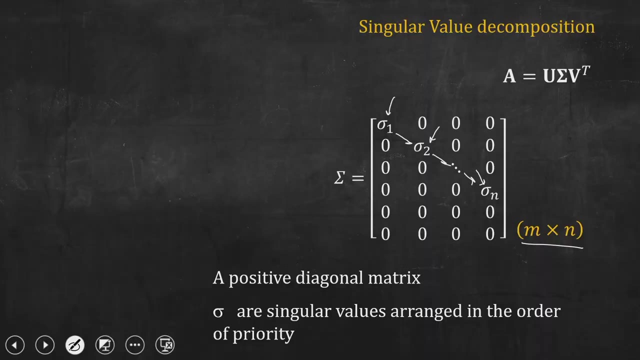 sigma 2 up to sigma n right. these are small sigma and as it is a rectangular matrix, obviously i will have to put the it use the diagonal, the main diagonal of the rectangular matrix. so i have these values along these main diagonal and rest of the values are zero. rest of the. 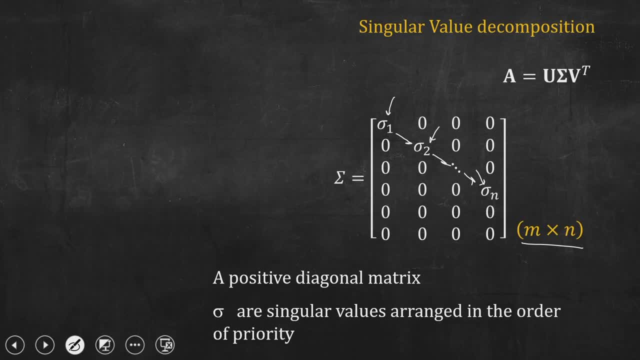 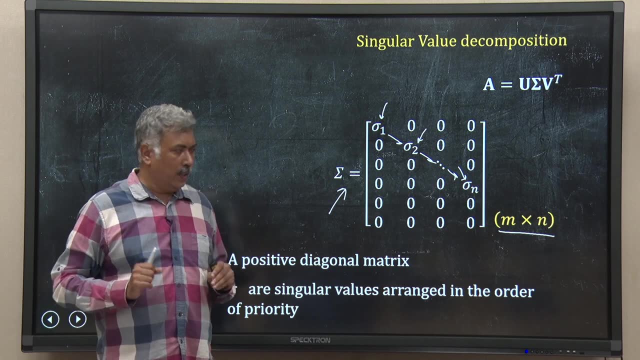 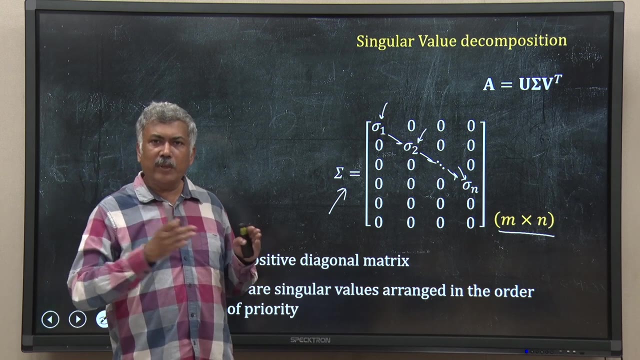 values are zero, right? one important thing in this case we have to remember: we want that this is a positive matrix. that means all these sigma values that i have written right e are positive values. fine, so this is one constraint we are putting and also what we do, just like in case of arrangement. 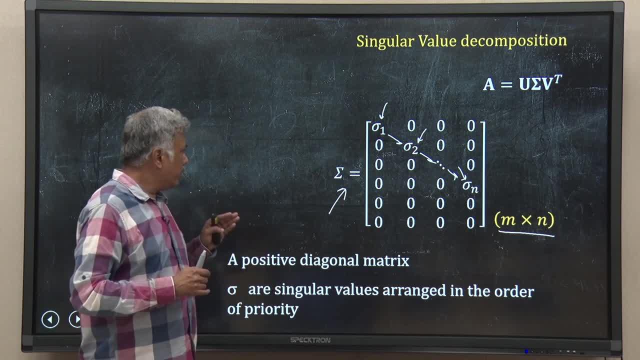 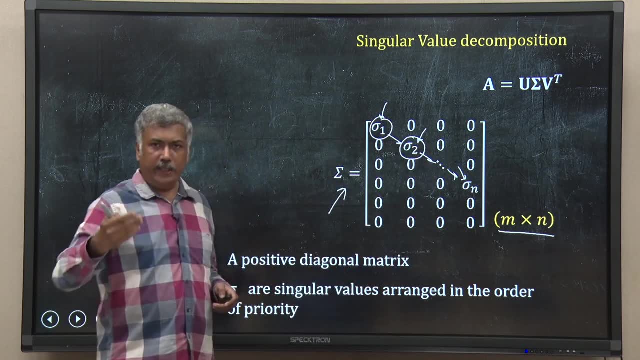 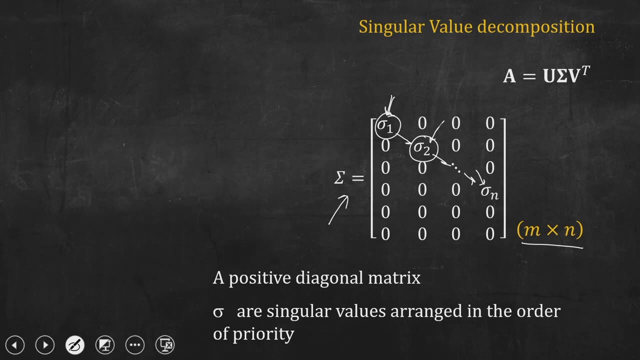 of eigenvalues in eigen decomposition. we usually in that analysis, what we do? we arrange this term sigmas in order of priority. that means i will put the highest positive value first, that will be sigma 1, and next the second value will be sigma 2, the right, and this will be. 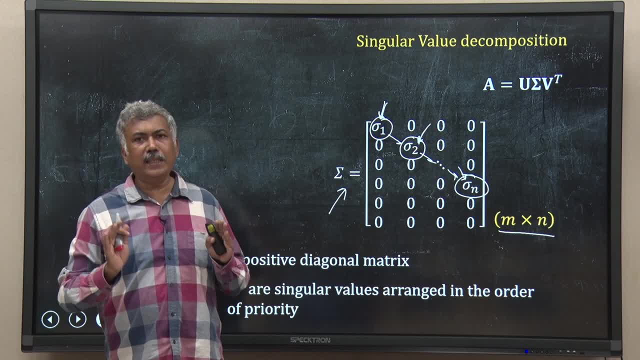 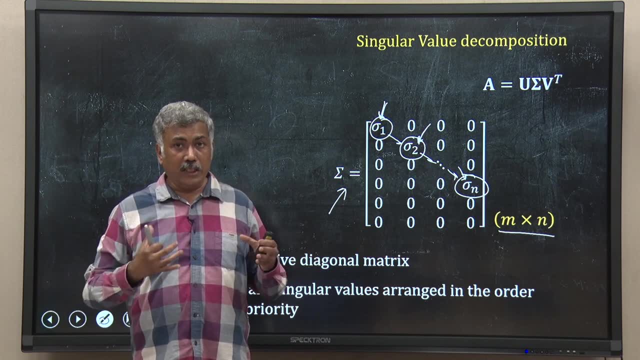 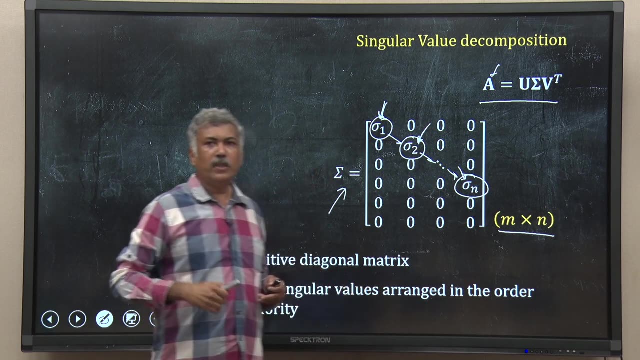 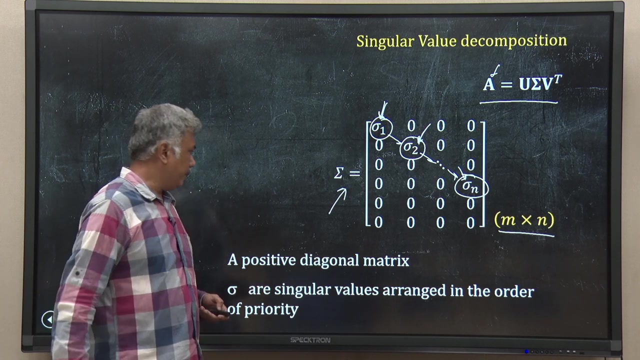 the lowest non-zero value. right like that. we arrange it in this way, right? so i have defined u, v and sigma and i want them in such a way that i will. if i combine them in this particular form, i will get a right. so, in other words, if i break, decompose a, i should get u, sigma and v transpose. 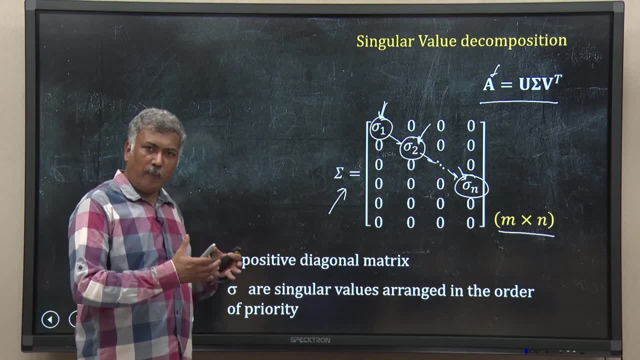 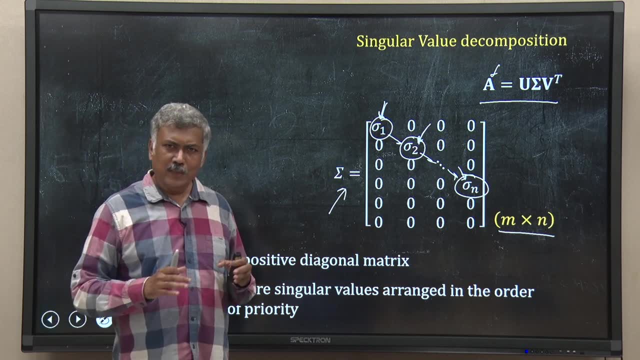 so now comes the question. that is my wish and i have defined these properties: there will be orthonormal, they will be diagonal matrix, right. but how should i get those u, v and sigma? that is not very difficult. this is a straight forward linear algebra method. i will show part of 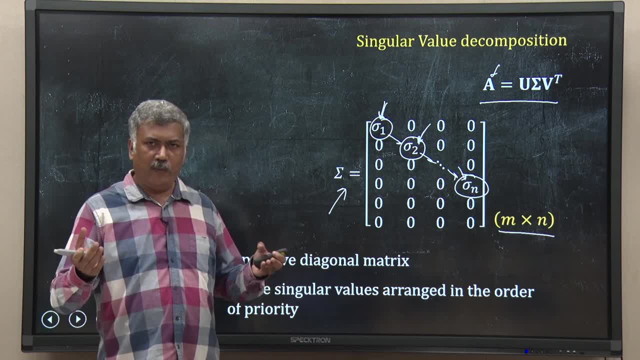 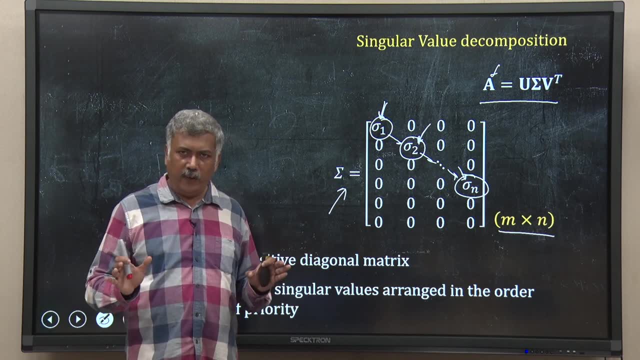 it and i will skip some steps. if you are interested you can do it yourself also. maybe here and there you have may have to consult a linear algebra text somewhere to know some rules, but otherwise it is not so difficult. but for this course you do not need to go into detail. 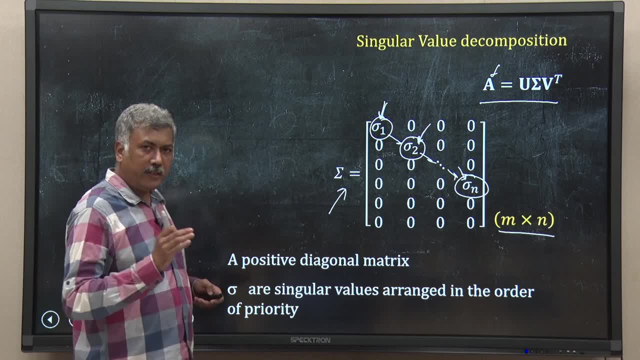 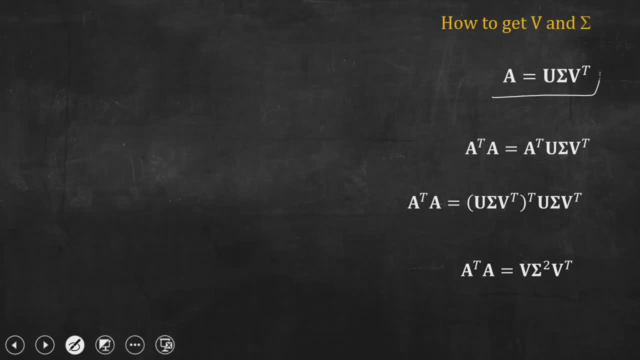 of the proofs either. so let us start and see the logic and try to understand the logic right. so we have to calculate v and sigma. so i have this relationship right. that is my i want. so multiply both side of the equation with a transpose. so i multiplied this side also. 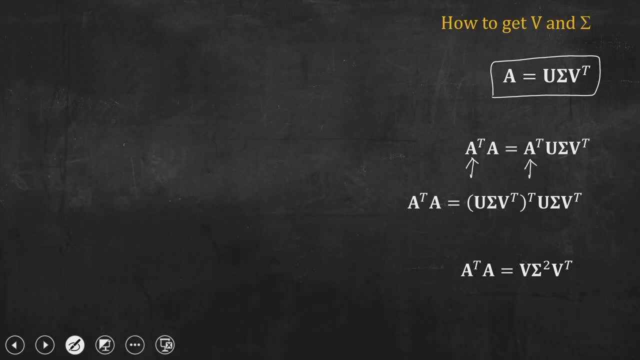 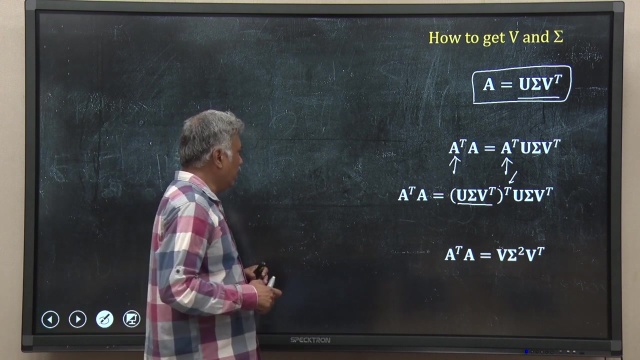 with a transpose. now, what is a? a? by my definition is u sigma v transpose. so i put u sigma v transpose and i transpose the whole thing. and now in this step i have skipped lots of steps. if you want, you can check it out. so, after multiple step of using linear algebra rules, you will land. 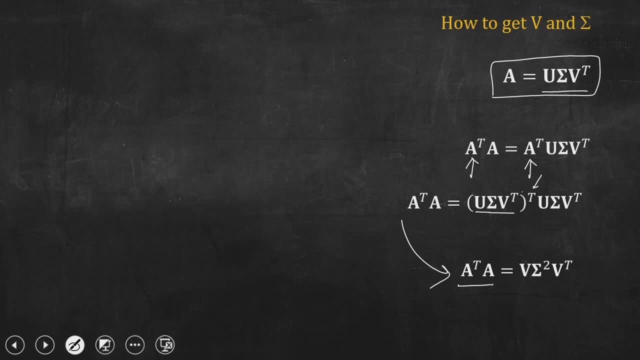 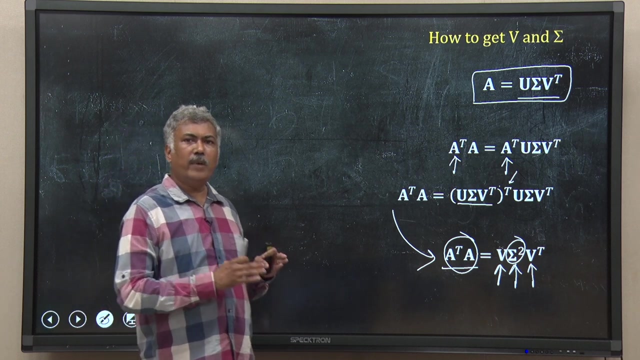 up into this relation. a transpose- a is equal to v- into sigma square, v transpose. i will discuss what is sigma square and what is a transpose a is meaning r, so i will get a transpose a right. so you are multiplying the transpose of a matrix with a on the that is, on the left. 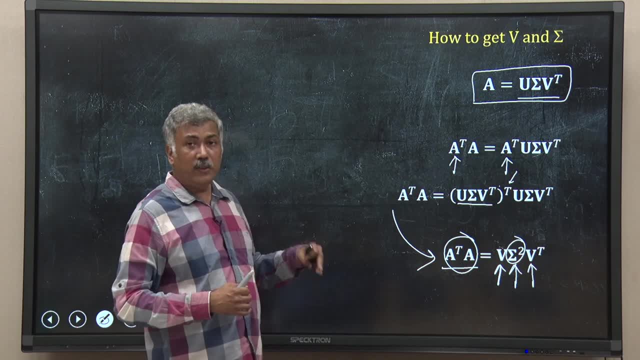 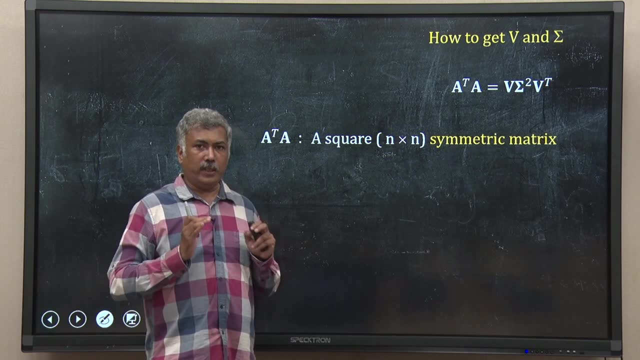 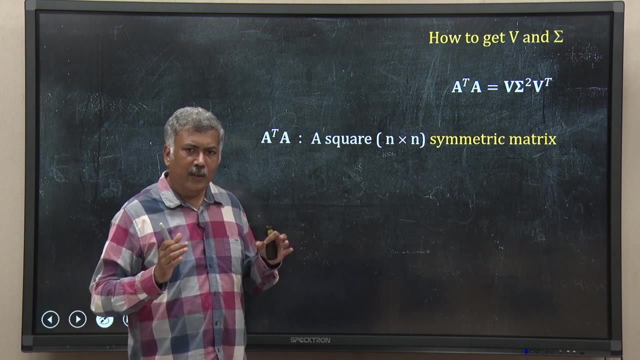 hand side, on the right hand side. what you have got? you have got a v, v into sigma square and v transpose. so now look into a: transpose a and its properties. just like magic of linear algebra, a transpose a, whatever matrix you take, a you will have. 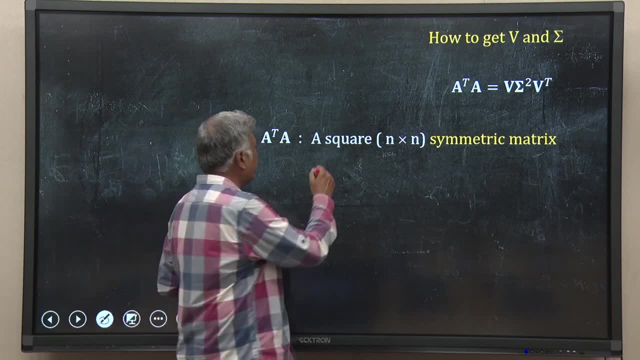 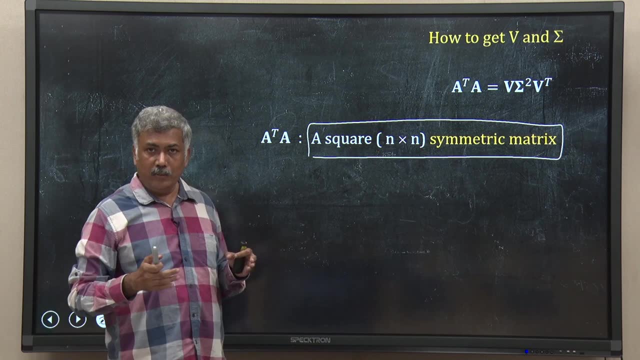 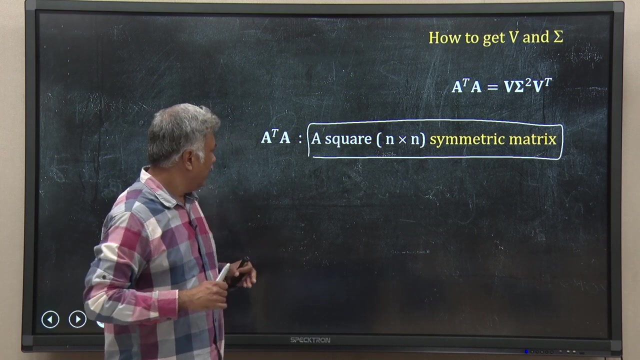 a very interesting property. a transpose a will be a square symmetric matrix. right, it will be square matrix because you started- you may have started- with a rectangular matrix, but when you multiply with this transpose, you will eventually land up with a square matrix. so you have a square symmetric matrix. 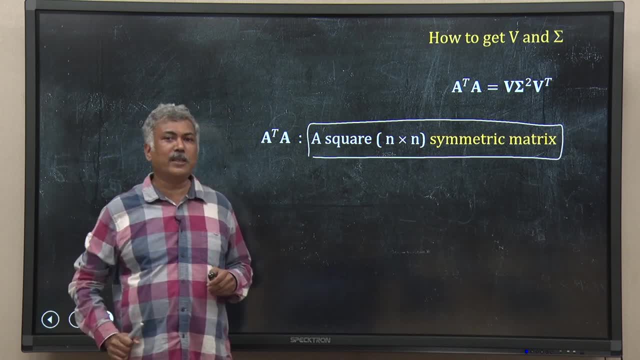 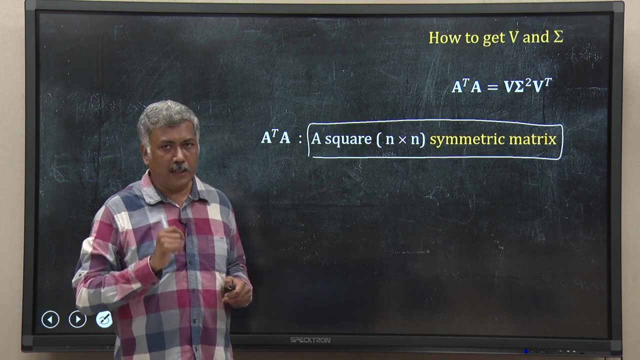 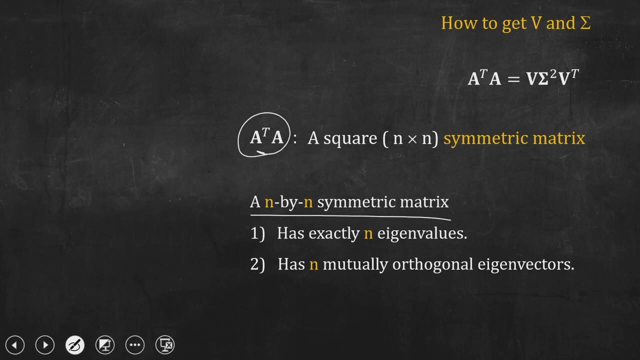 now, if you remember from our eigenvalue eigenvector discussion, symmetric matrix has a very interesting property in terms of eigenvalue and eigenvector. what is that? just to remind you, if i have a n by n symmetric matrix like this one, then we have discussed in the eigenvalue lecture. 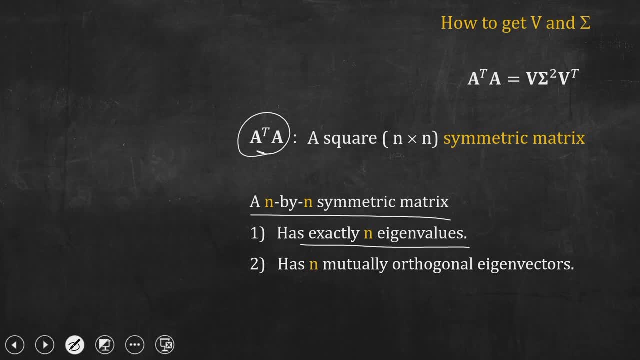 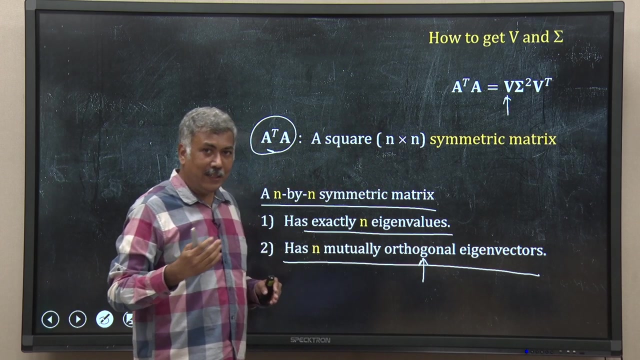 is that it will have exactly n values and it will have n mutually orthogonal eigenvectors. so i will get n mutually orthogonal eigenvector- pay attention to this issue- orthogonal, remember. i want the vectors in this capital v should be orthonormal, right? so one requirement is that the vectors has to be orthogonal. normalization: 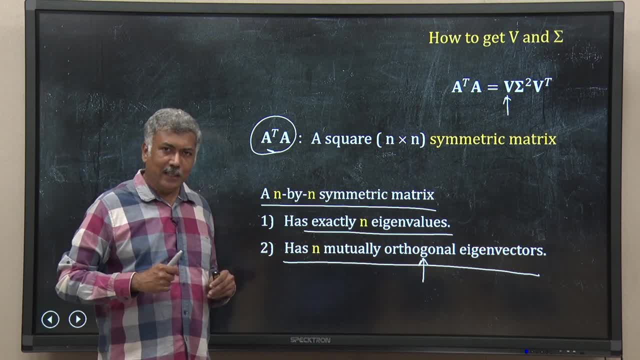 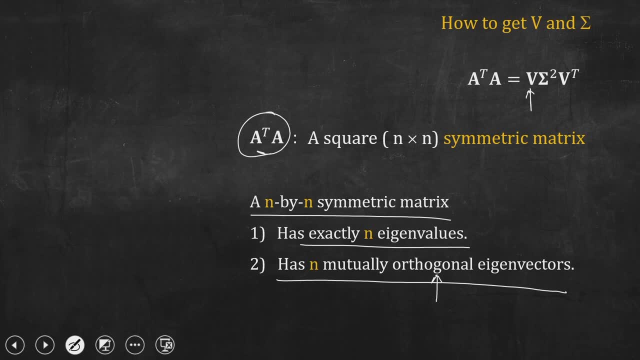 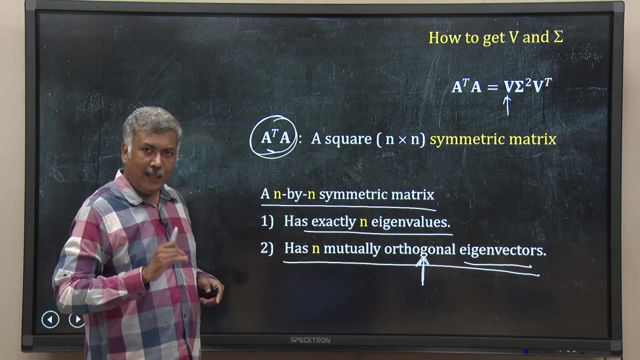 you can always do of any dividing it by length. So the first priority is, obviously you may need to be orthogonal, and we are moving towards that, that A transpose A will have eigenvectors and those eigenvectors will be orthogonal. Let us move into sigma square. sigma square. 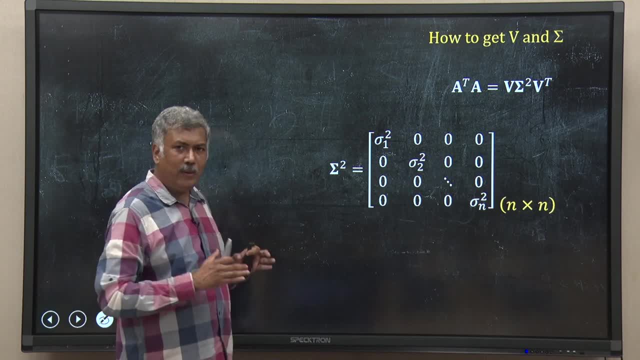 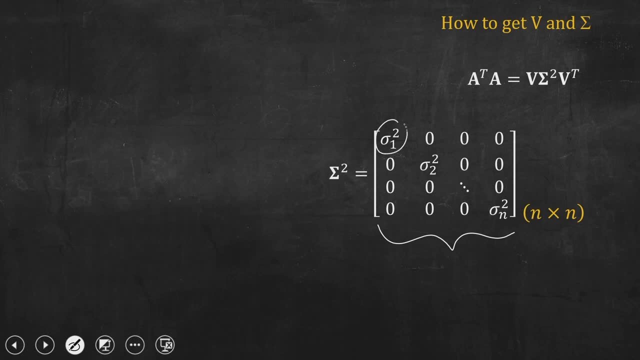 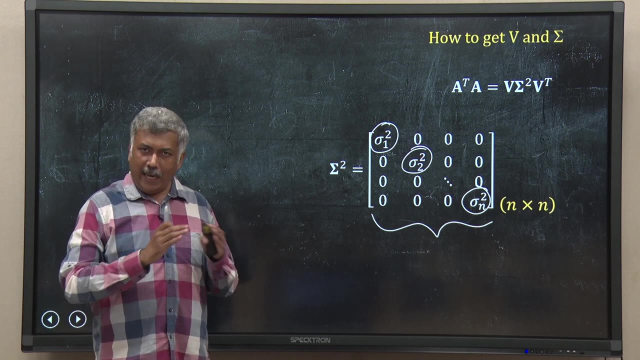 here in this calculation, if you do the derivation, you will find the sigma square. you will land up of this form: It will be n by n, diagonal matrix with diagonal term sigma 1 square, sigma 2 square and sigma n square. So it will be n by n square matrix, diagonal with. 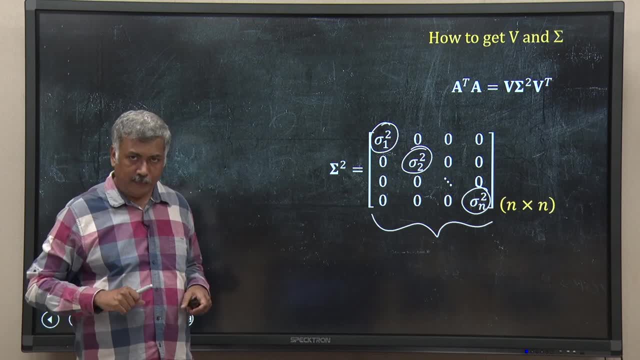 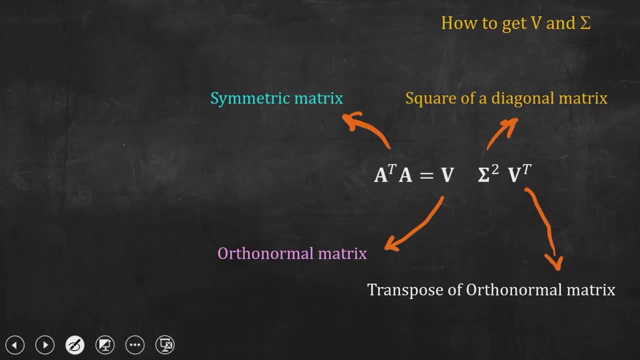 the sigma terms along the diagonal in the square form. So let me rewrite the whole scheme. what do I have? I have A transpose A that is equal to V into sigma square, into V. transpose A. transpose A is a symmetric square matrix, V is a orthonormal matrix. that we want, We defined it that way and I am calculating V. 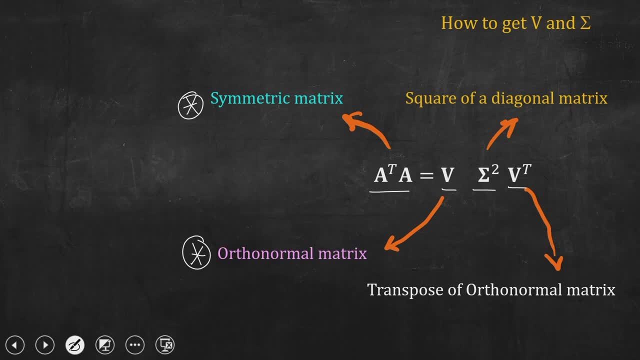 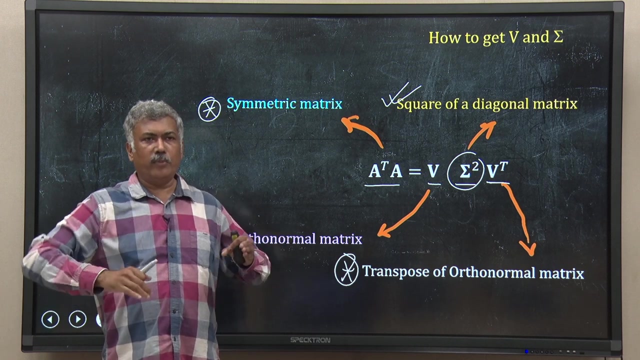 I am trying to find out V. What is V transpose? V transpose is transpose of that orthonormal matrix and this sigma square is nothing but a square of a diagonal matrix. Remember, if I give you a diagonal matrix, So suppose, 2 by 2, it has A and B along the diagonal. 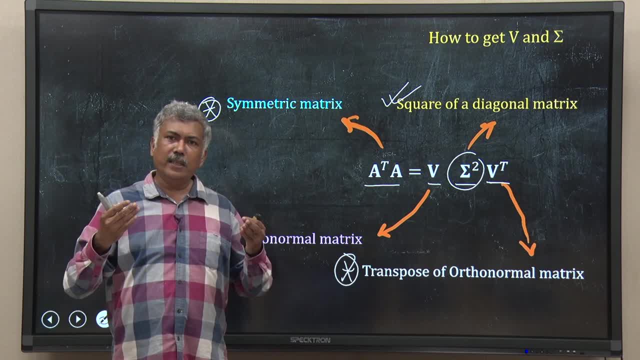 So if I write the diagonal matrix, I would give the sigma square and ë0 ë partially 49, is equal to ë1 ë drive, ë1 ë and ë 0, ë само, ë, other parts. 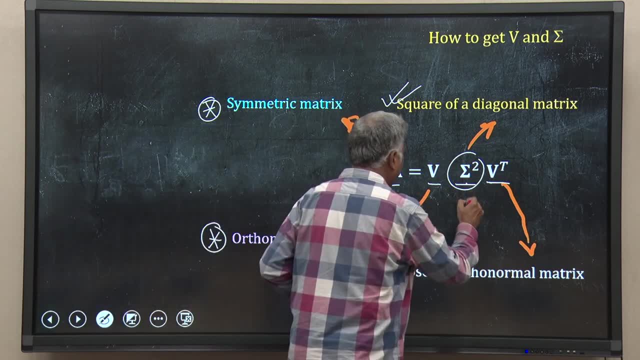 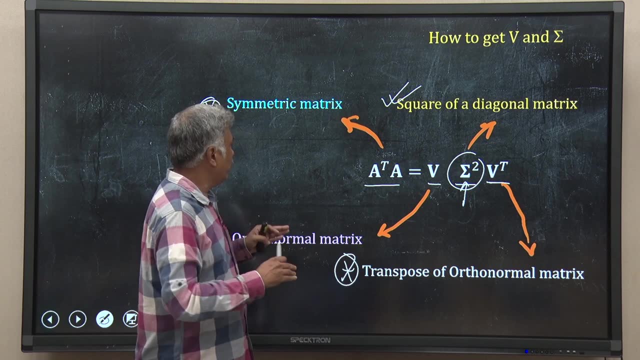 If you square it, you a. it is very simple. The diagonal terms will get multiplied. So I can say: sigma is nothing but a diagonal matrix. So is sigma square is also the square of the terms of the diagonal matrix, right. So sigma square, justice, square of a diagonal. 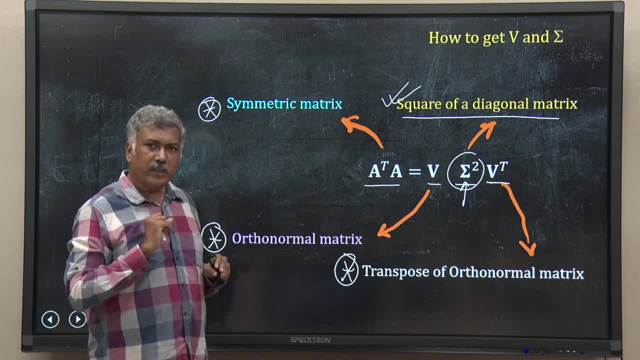 matrix. Now there is the very interesting property in linear algebra- and that will save us in this derivation. It is known, or rather it can be shown that it is known- The very interesting property which is known by k and n in head. Karena senor, is it that îf- to скорiss night? 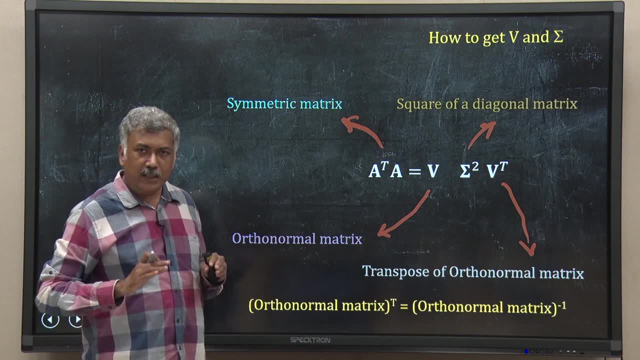 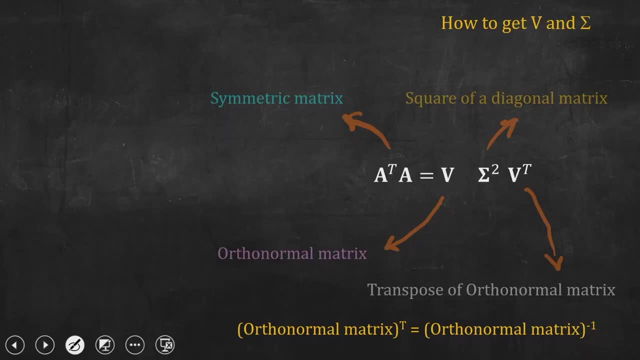 è3r is Analytics accordance of n which supportive to virtually God53, to the Single hypothesis, The that for an orthonormal matrix. That means a matrix made up of vectors, column vectors, which are orthonormal. If I have an orthonormal matrix, its transpose is same as its inverse. 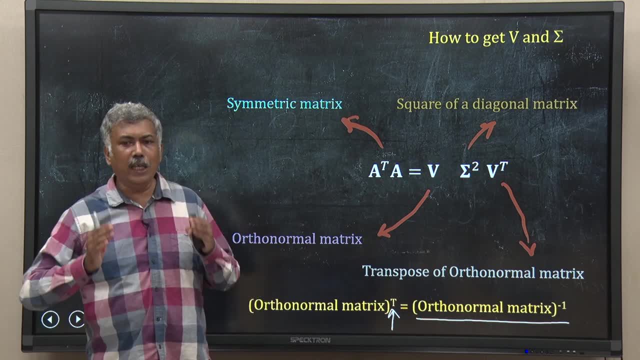 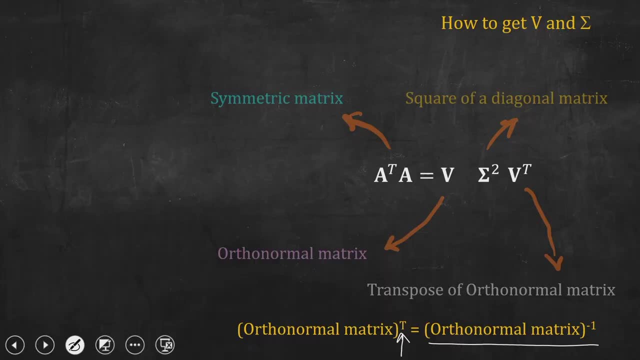 So the transpose of an orthonormal matrix is equal to the inverse of that matrix. So what I can do here, I can replace this transpose by inverse. So I can write A transpose A equal to V into sigma square, into V inverse. I can write that. So that is what I have. 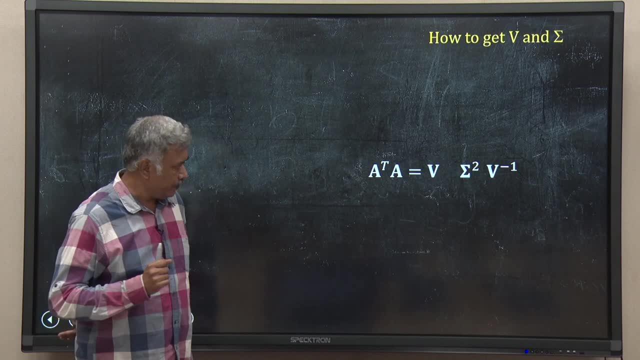 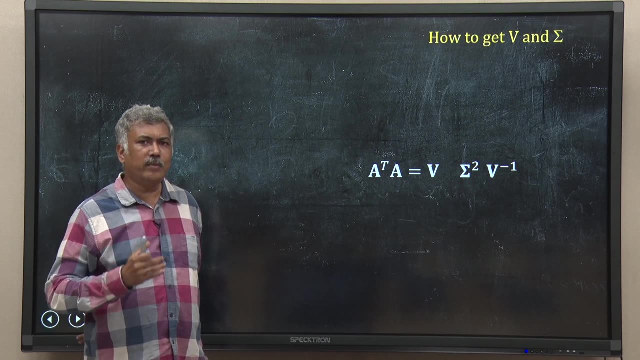 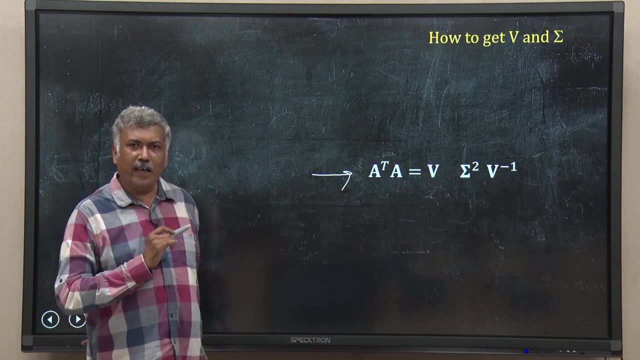 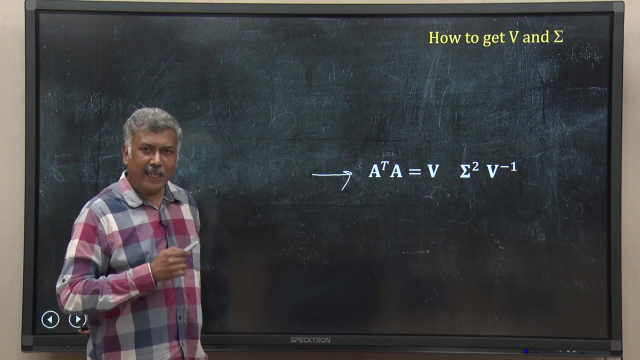 written. Pay attention to this relationship. Do you find something hidden in this Some relationship that we have discussed a few minutes back, hidden in this particular structure? If you pay attention, you will find this has a similarity. This is the similarity with eigendecomposition. Let me show that. Let me write: eigendecomposition. 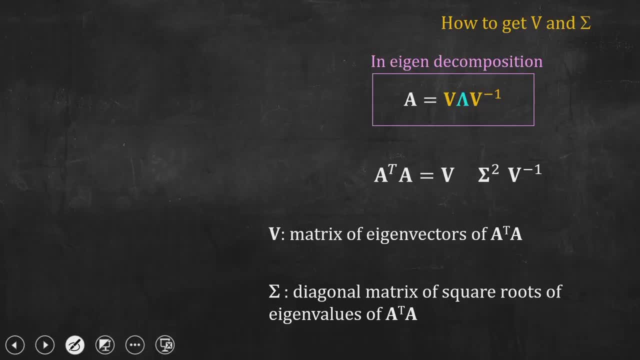 form. So in eigendecomposition, what I have done, A is equal to eigenvector matrix into my lambda matrix, the eigenvalue matrix and the inverse of the eigenvector matrix. That is what eigendecomposition Now imagine. A transpose, A is same as A. So this is the 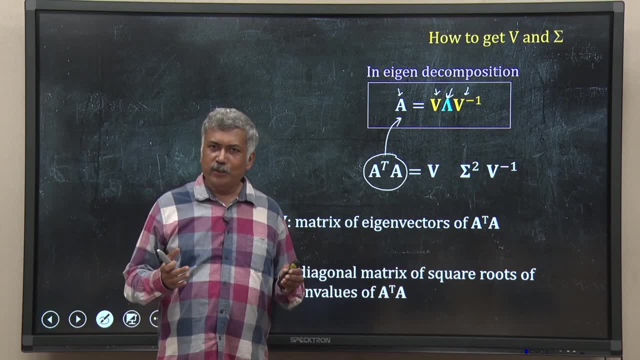 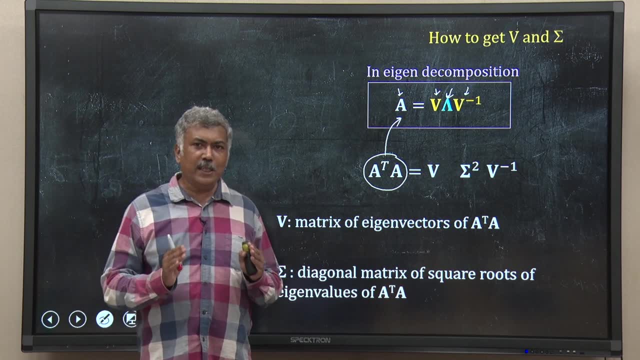 vector A. You can see that. You can see that it is a ϱ- Salv. A transpose: A is a ϱ- Salv matrix, So it can have eigenvalue. eigenvector A is a rectangular matrix. I cannot have eigenvalue. 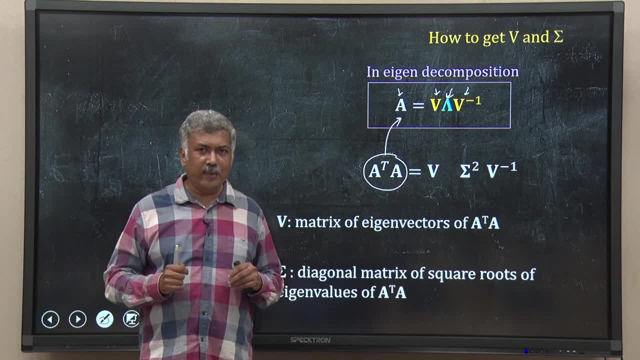 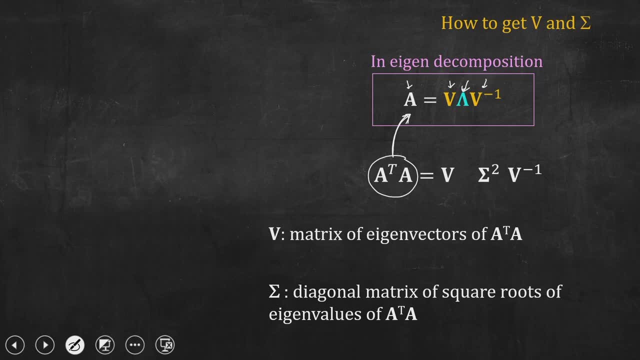 eigenvector for that. But A transpose A is a square matrix, a square symmetric matrix. It can have eigenvalues, eigenvectors. So this is A, suppose this is A, Then I can map them. So this V is this V, this V inverse is this V inverse. and this sigma square is: 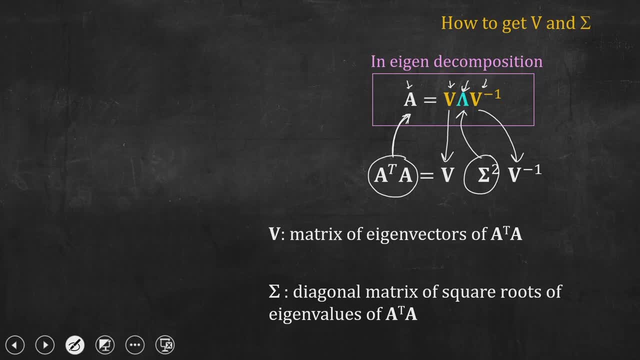 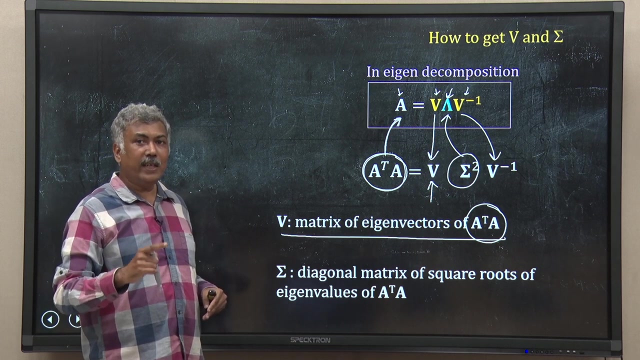 1 to 1 correspondence is there. So that means if I consider these as a single matrix, obviously it is a single matrix. then, on the right hand side, what do I have? I have a matrix of eigenvectors of A transpose A. And remember, A transpose A is a symmetric matrix, So its eigenvectors. 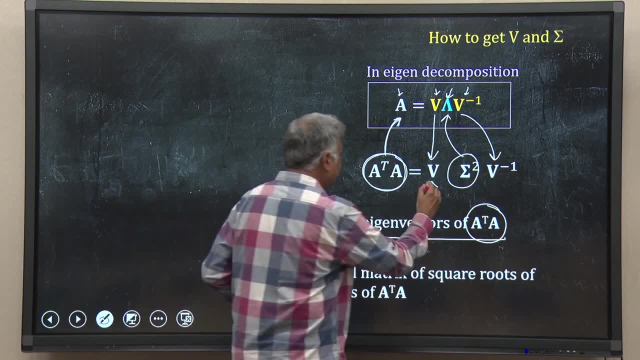 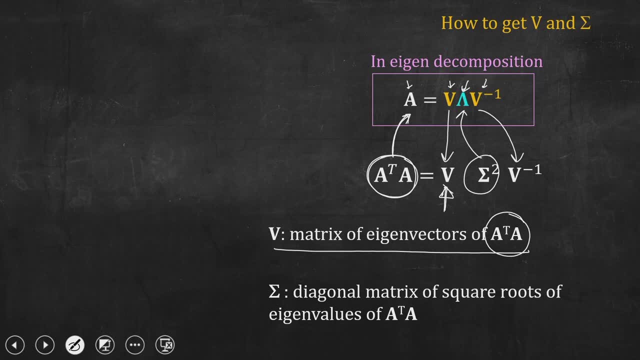 are orthogonal, and that is what we want. So this is a matrix square, matrix of vectors which are orthonormal. Similarly, this will be the just the inverse of that one, And this sigma, this sigma square, is a diagonal matrix right, And this is also a diagonal matrix. 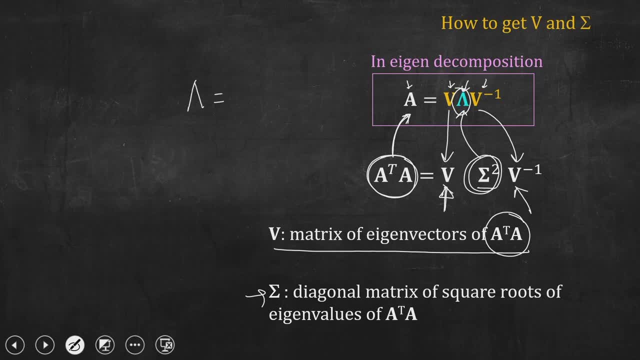 So in case of lambda, what I have I have, suppose, if I take 2 by 2, lambda 2 by 2.. So lambda 2, 0, 0.. And for sigma square, if I have sigma one square 0, 0, sigma 2 square, 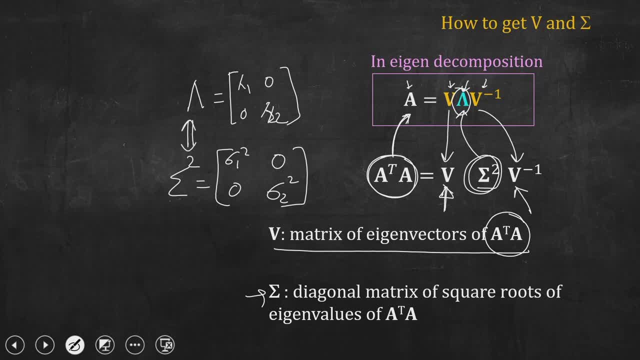 Then if these two things are equal, then lambda is nothing but sigma one square. lambda two is nothing but sigma two square. Now what is lambda 1 and lambda 2?? lambda 1 and lambda, the two are now the eigenvalue of this. A transpose A, So sigma is the diagonal matrix of square. 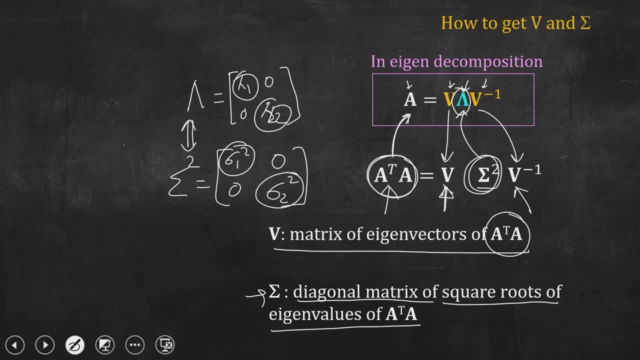 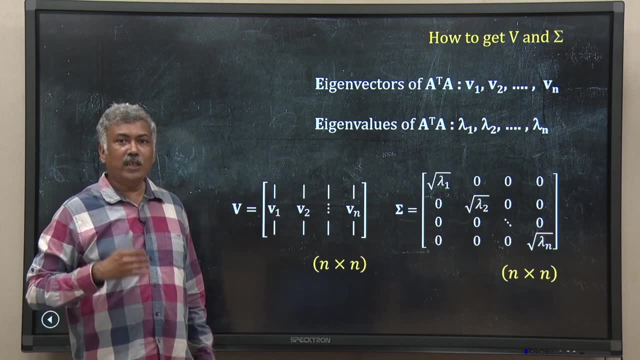 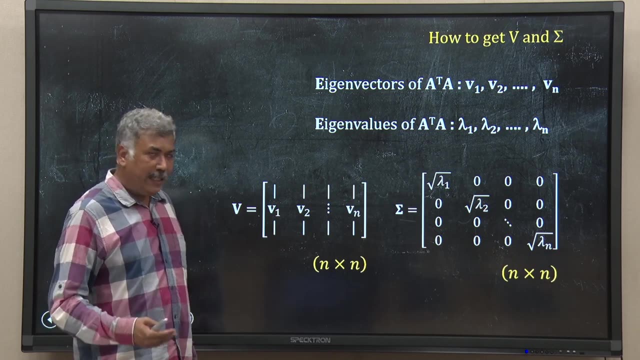 roots of eigenvalues of A, transpose A- That is what I have got- and calculate an eigenvalue eigenvector we know. So if you give me a rectangular matrix, general matrix A, then what I can do is that, as I am doing eigen decomposition, I have to calculate V and sigma. 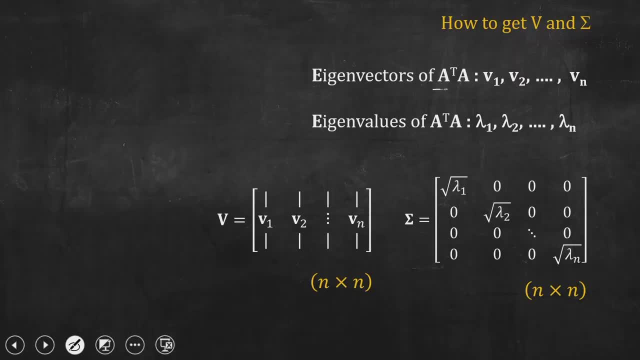 So I will calculate the eigenvectors of A transpose A and suppose they are V1, V2 up to Vn, and the corresponding eigenvalues of A transpose A are lambda 1, lambda 2 and lambda n, Then the V matrix is a square matrix, for my SVD will be V1, the first eigenvector. second, 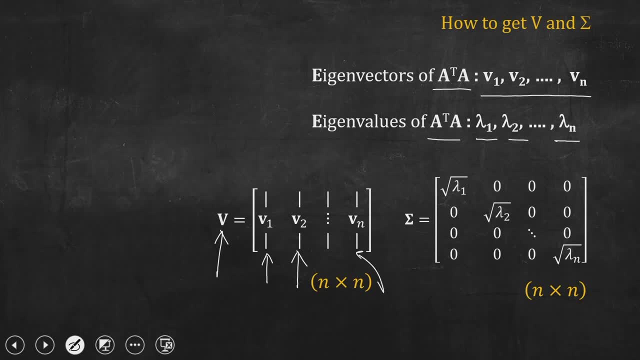 eigenvector third, and so the nth eigenvector, Whereas the sigma will have the square root of the eigenvalues lambda 1's root, lambda 2's root, up to the square root of lambda n, the nth eigenvalue of A. transpose A As I. 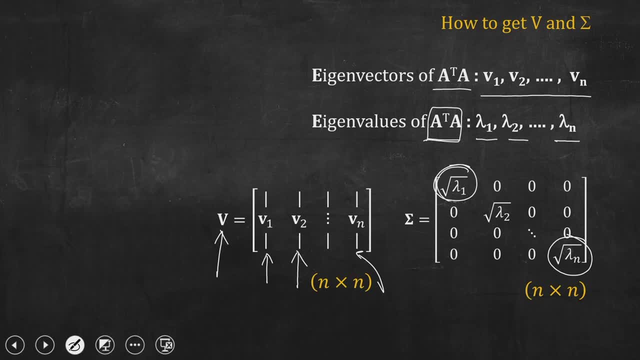 said by convention, what we do, we take the largest value here, second largest value here, and then the other, in the order of priority. Similarly so this one is the largest value. one will be corresponding. the first vector will be corresponding to lambda 1, second. 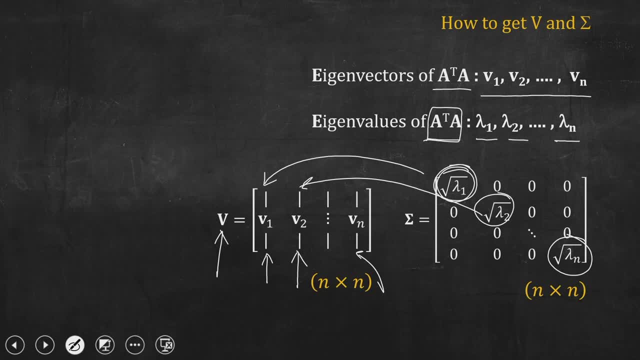 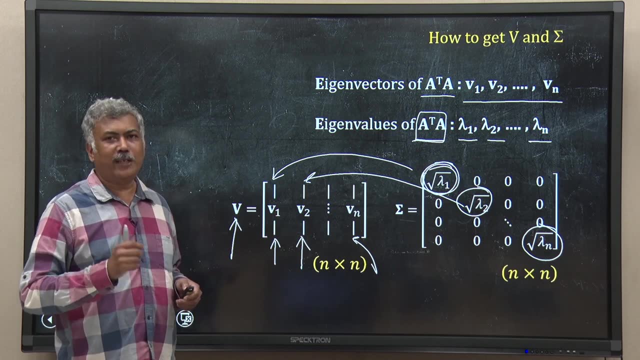 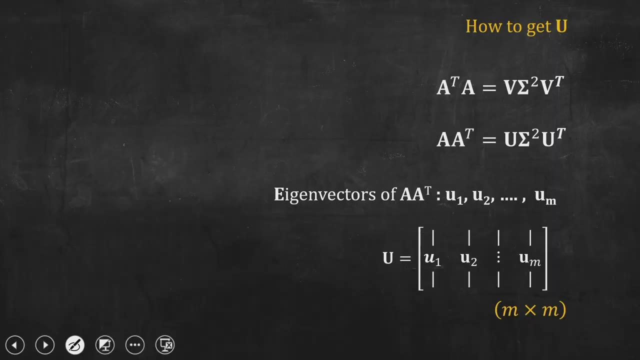 one will be corresponding to the second Eigen value. This way we arrange them. So I have got V and sigma. I can use actually the similar technique for to get U. I will not go into the derivation of how we get U, just I will show in one line. So I have got V by taking 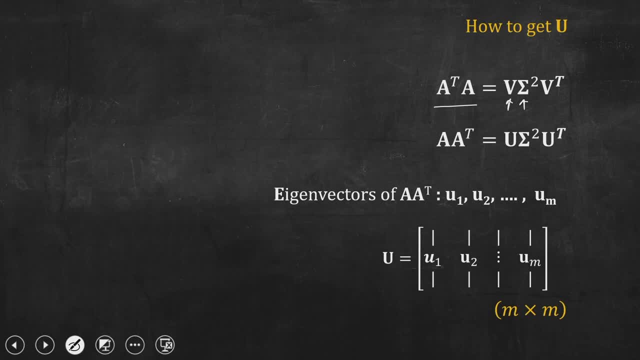 A transpose A, and that gives me V and sigma square. And if I do A into A transpose, just the opposite one: A into A transpose, I will get U sigma square, U transpose, I will get this relationship. So what is U now? U is the Eigen vectors or matrix of Eigen vectors. 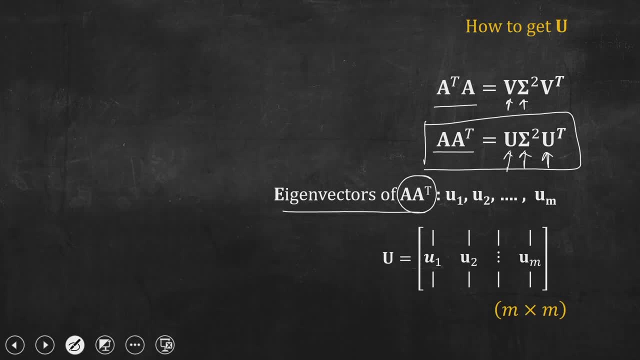 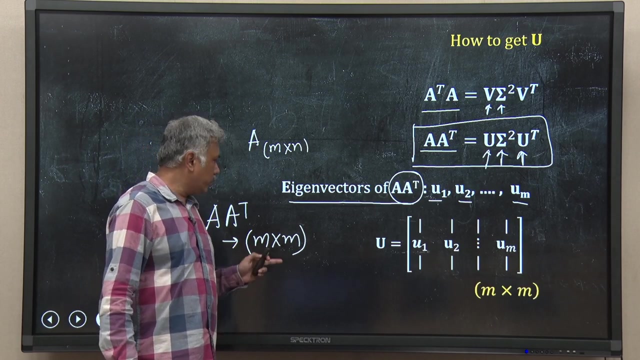 of A A transpose. So they are U 1, U 2 up to U m. Remember, if I have A is m into n matrix, then A into A transpose will be of m into m dimension. So that means it should, it will be again a symmetric matrix. So it should. 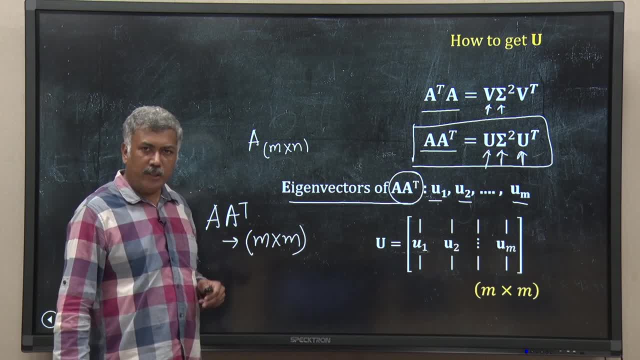 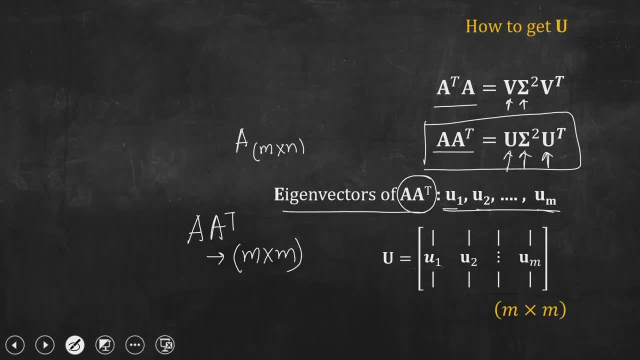 have m Eigen values and m Eigen vectors. Each of these Eigen vectors will be orthogonal to each other. So I have U 1, U 2, U m. All these are orthogonal Eigen vectors of A A transpose and I have stacked them together side by side to get a M by M matrix which 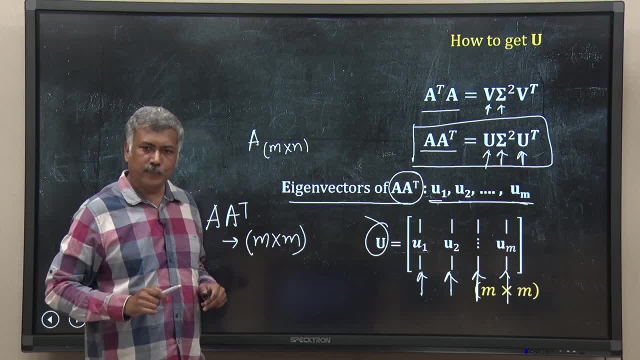 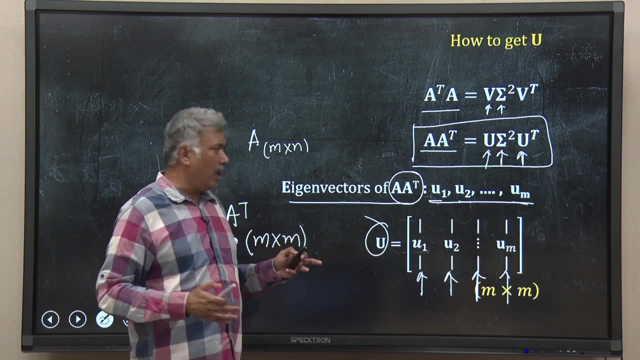 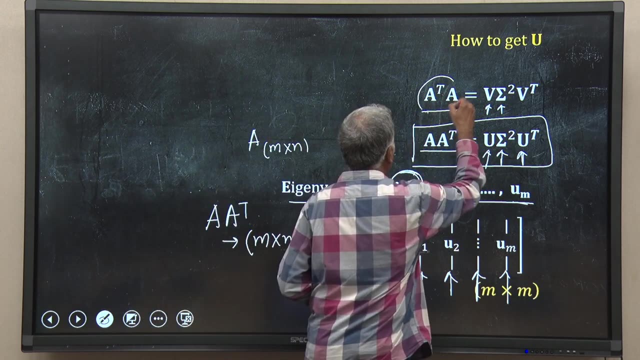 is my capital U matrix in SVD, The Eigen values. if you look into it- you can try yourself or look into the textbook- you will find the Eigen values of A. A transpose will be same for non zero values, for the Eigen values of A transpose A. So for these two things, the Eigen values. 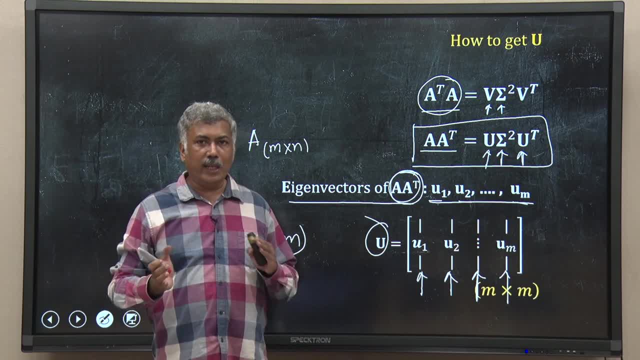 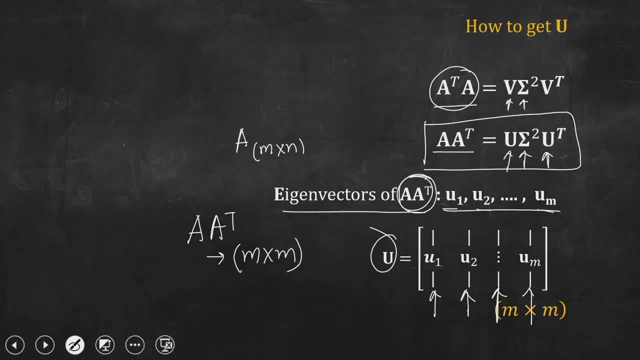 non zero. Eigen values are same, only there will be some Eigen values extra in one case, depending upon the value of M and N, which will be 0. right, because the dimension has to be matched, because this is M into M. in the other case, it was N into N, So non zero. 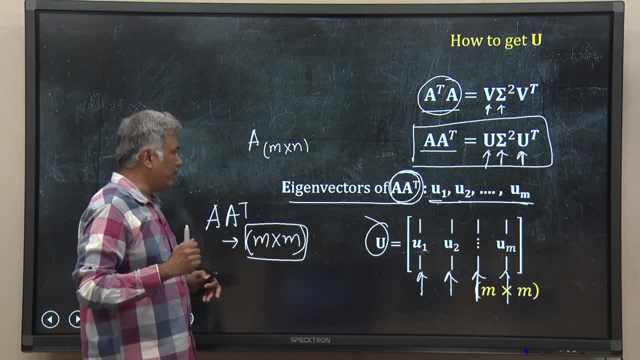 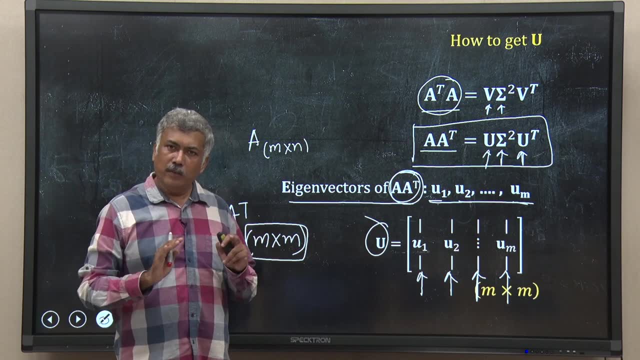 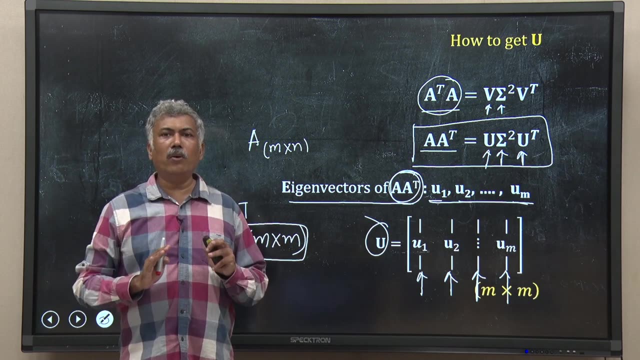 terms will be same. zero terms will be extra zeros or less zero will be there, depending upon the relation between M and N. So I, what I have got, I have got V, I have got sigma, I have got U. So now I go back and represent the whole SVD in one slide. What I am doing, I have 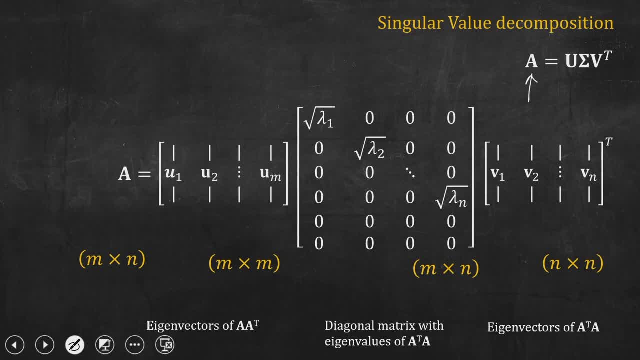 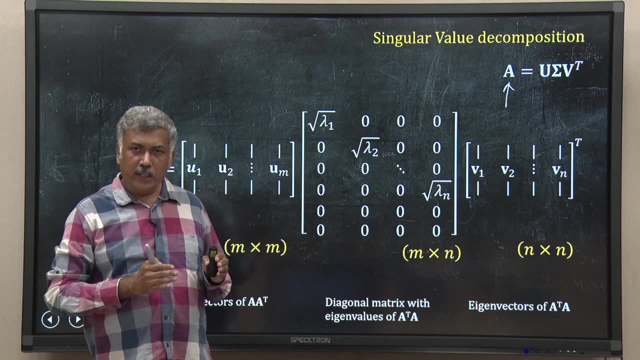 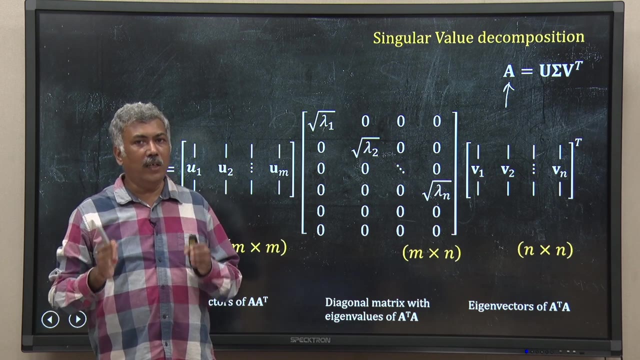 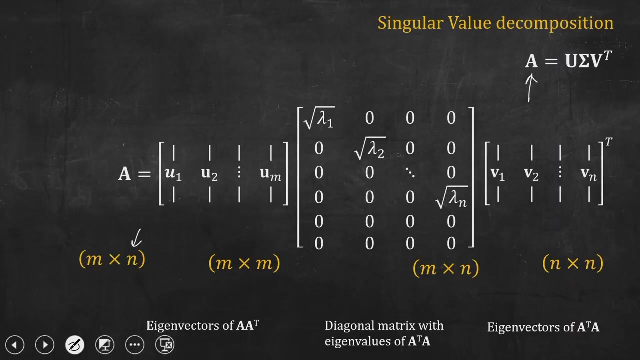 a M into N, a generalized rectangular matrix, A, and I am decomposing in it into three component: A U matrix, which is square, A sigmas matrix and A V transpose, which is also square matrix. So what do I have? A is M by N. I have this U matrix, which is M into M, and the elements here are the Eigen. 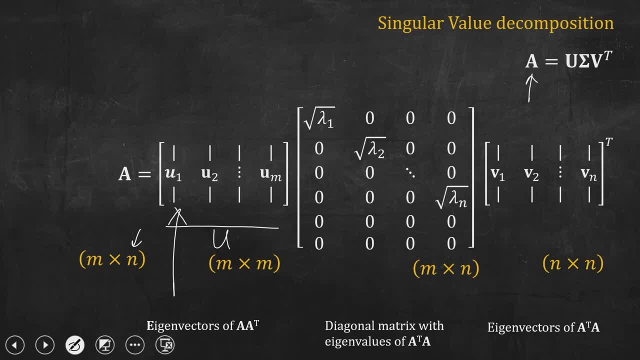 vectors of A A transpose, Whereas this one is my V matrix, having M into N the size and is Eigen. these vectors are nothing but Eigen. vectors of A transpose A. features are nothing but Eigen. vectors of A transpose A Cool. So that is what I am doing: I am removing, it. I will Guan C by cuts. I am going to equal to creepy grosso of what are these scene? That actually is the总 time, which is equal to 1 minus 2 by 2. Y to the W, the tangent. here we are just going to grocery, So here, in sum of you are all解. at Y, then, for complementing. 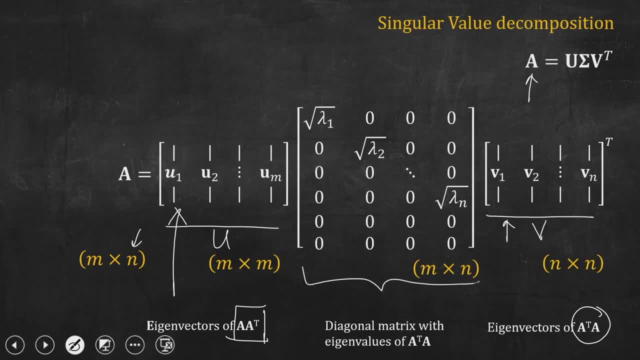 Y is 3M, the Fang閃 which is, according to that norm, d at the one filling in Y, never used forward. In the middle I have a m into n matrix where I have the eigenvalues, square root of those eigenvalues of A, transpose A, arranged along the main diagonal. So lambda 1,, lambda 2,. 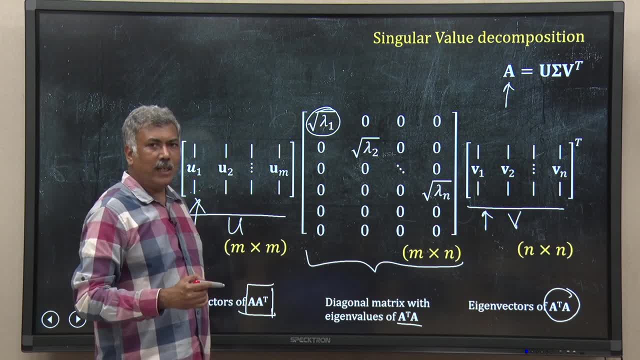 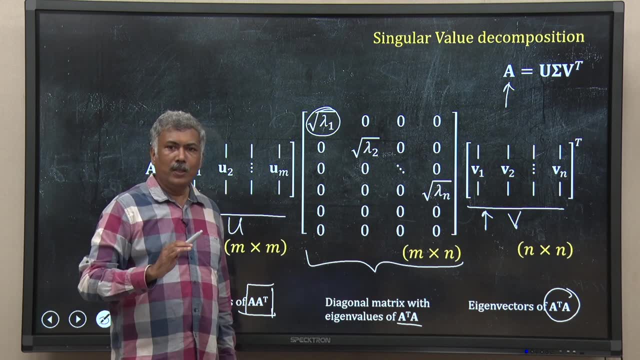 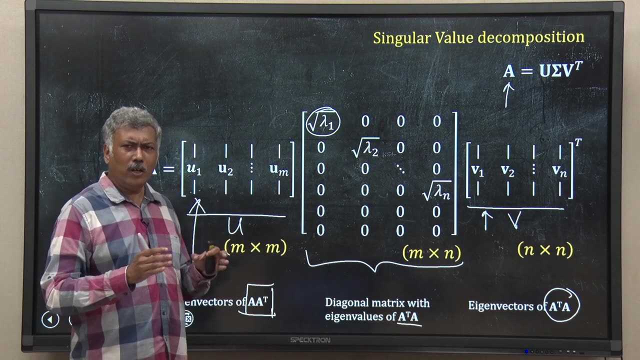 lambda n are the eigenvalues of A, transpose A, and we have taken the square root of that and we have arranged them along the main diagonal. So this is what we call singular value decomposition. There is something called economy size or economy SVD, What they do See, we have lots. 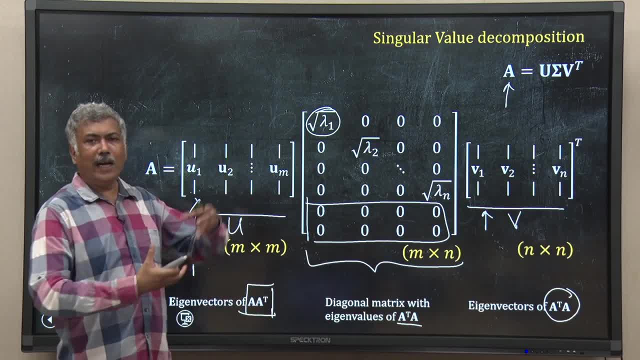 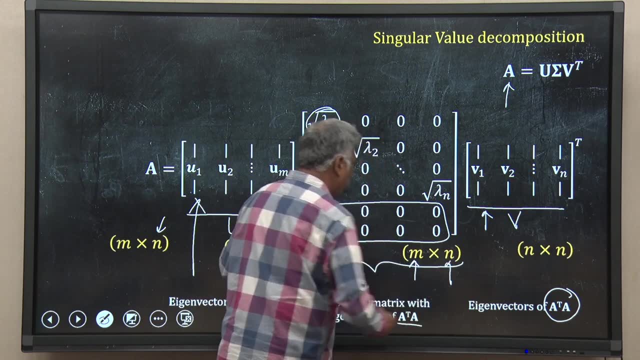 of zeros right here. and if you take a large dimension, suppose 2000 into 10 or something like that, then m is suppose 2000 and this is 10.. So you can imagine there will be lots of rows or lots of column. What way you do. 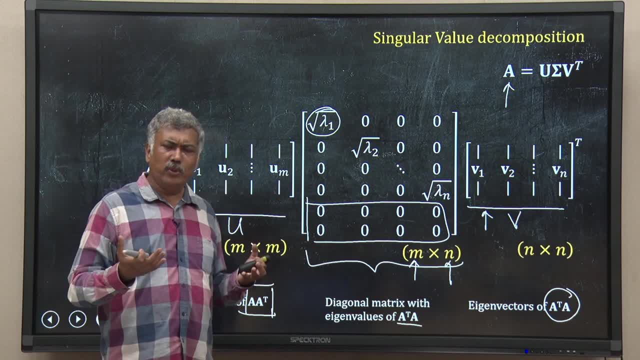 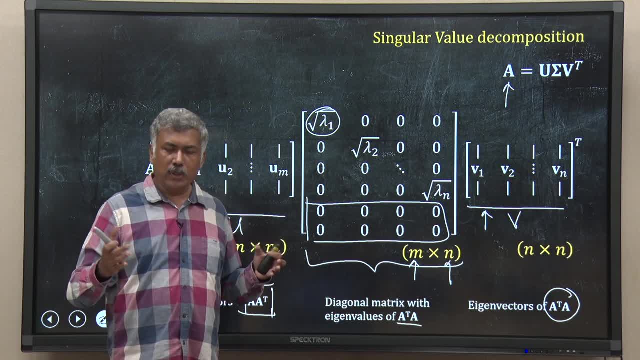 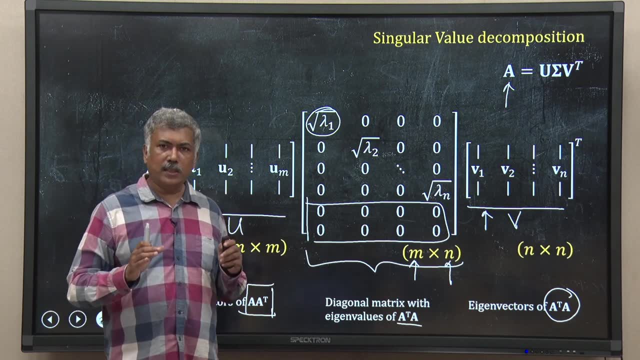 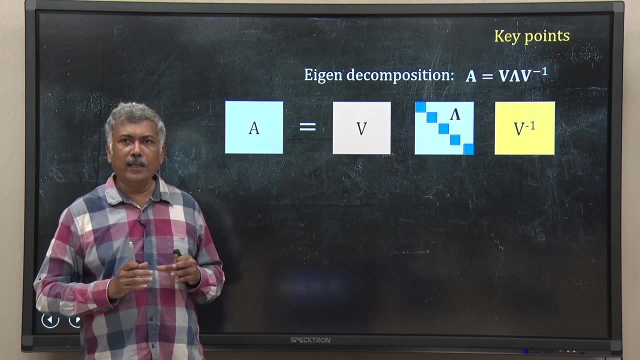 why many a time we chop those zero columns or zero rows and that is called economy size or economy SVD. So that is all for this singular value decomposition lecture. Let me jot down what we have learned In this lecture. the first thing we have learned is called eigendecomposition.